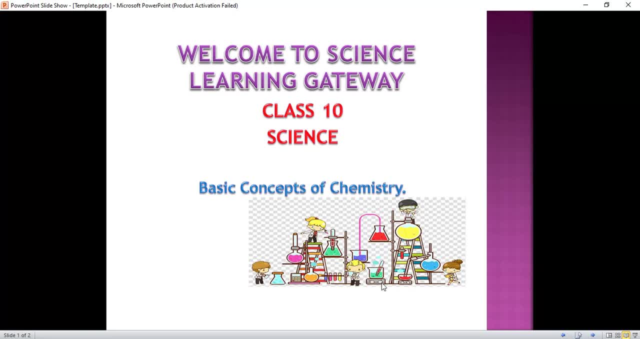 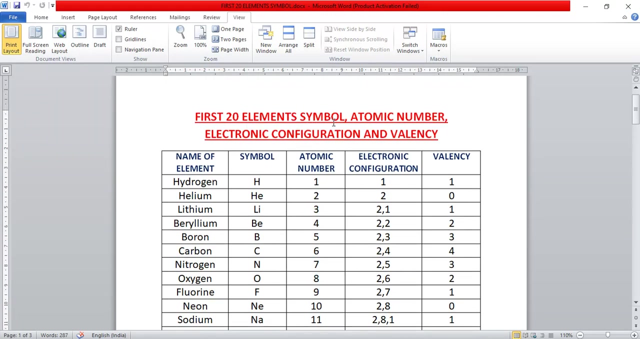 These things, the basic concepts of chemistry, which we will discuss today, will help you in your further studies. So you should learn those things and you should have a good concept about all the materials and the concepts. So let's start. First we will discuss about the first 20 elements: symbol, atomic number, electronic configuration and valency. 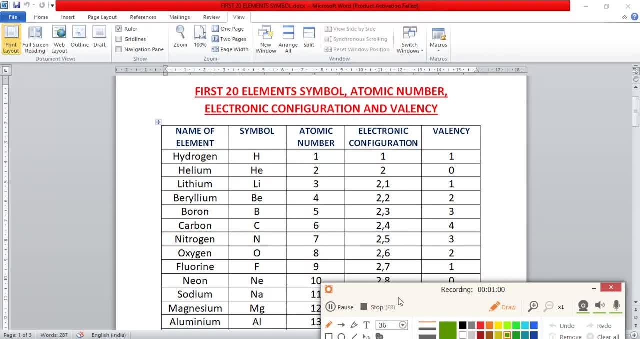 Let's start. Next element with atomic number 2 is helium. Helium has a symbol of He. We cannot give helium as a symbol of H, because hydrogen already has symbol H, So we have to give a different symbol to helium: helium, that is He. Third element with atomic number 3 is lithium with a symbol of Li. Fourth, 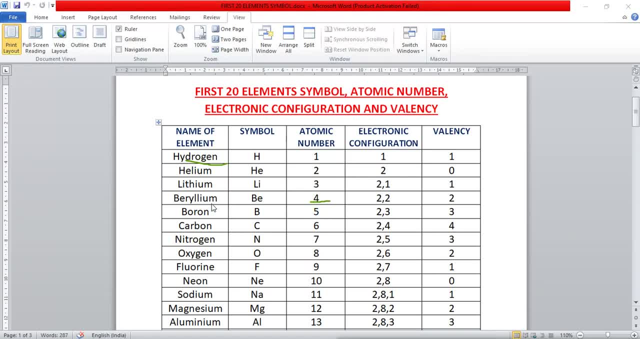 element with atomic number 4 is beryllium, and it has a symbol of B. Fifth element with atomic number 5 is boron, and boron has a symbol B. Sixth element, that is carbon. It has atomic number of 6.. Next element is nitrogen. Nitrogen has atomic number 7.. Eighth element is oxygen. Oxygen has 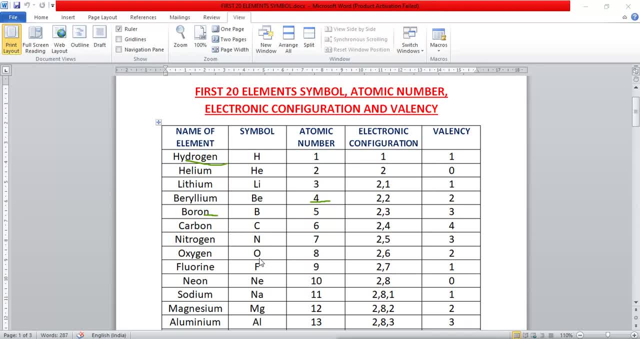 atomic number 8 and symbol is O- Fluorine- atomic number 9.. What is the symbol of fluorine F? Next element is neon. Neon has atomic number 10 and the symbol of neon is Ne. Next element is sodium. Sodium has atomic number 11 and the symbol of sodium is Ne. Next element is hydrogen Sodium. 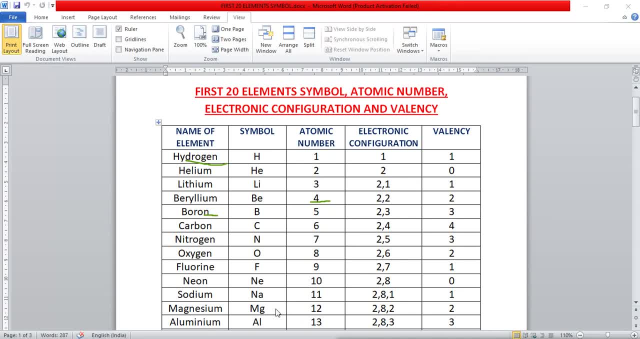 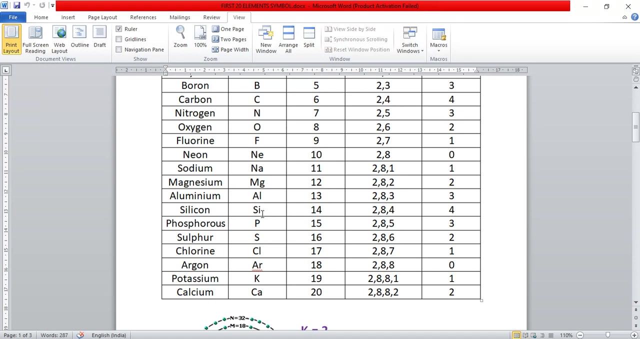 Na. Next element is magnesium: Magnesium. it has atomic number 12 and the symbol of magnesium is Mg. Next element is aluminium. What is symbol of aluminium? Al And atomic number of aluminium is 13.. Next element is silicon. Silicon has atomic number of 14 and the symbol of silicon is Si. 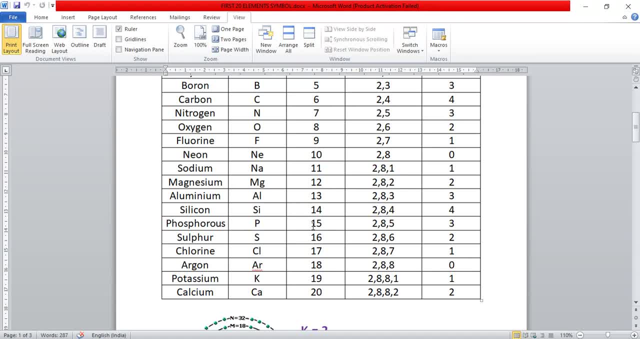 Next element is phosphorus. Phosphorus has atomic number 15.. Sulphur, with atomic number 16, has a symbol of X. Next element is chlorine. Chlorine has atomic number of 17.. Next element is argon. Argan has atomic number of 18 and the symbol of argan is ar. Potassium: Potassium has atomic. 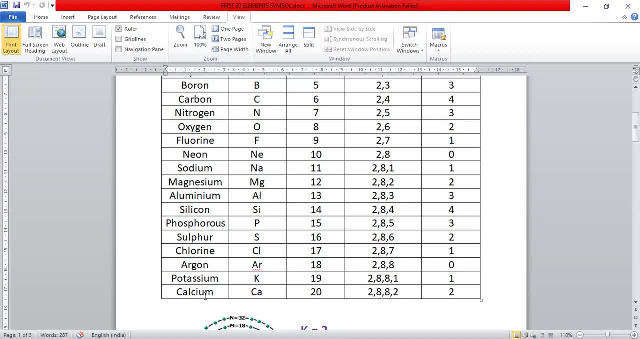 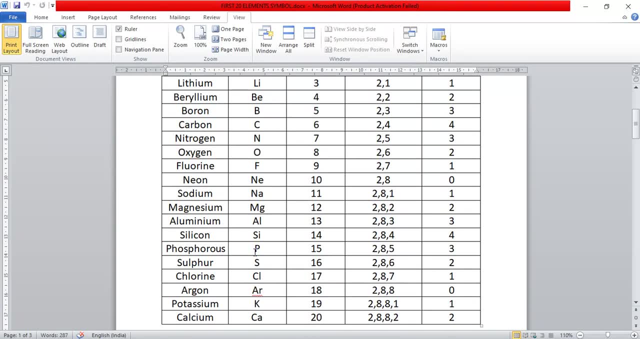 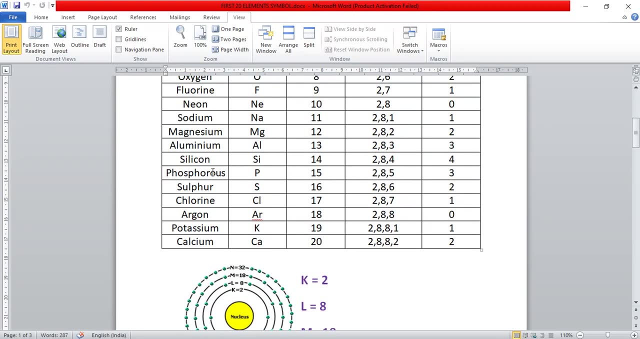 number 19 and the symbol of potassium is k. Next element is calcium. Calcium has atomic number of 20 and the symbol of calcium is ca. So these are the 20 elements, from hydrogen to calcium. You should remember the symbol of these elements because, without knowing the symbols of these, 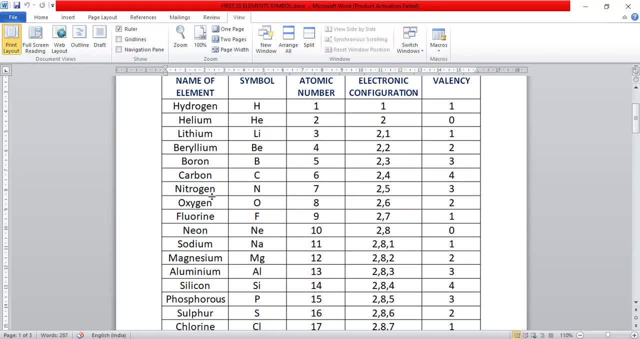 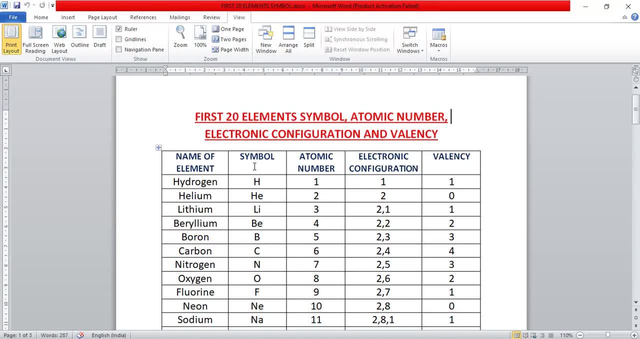 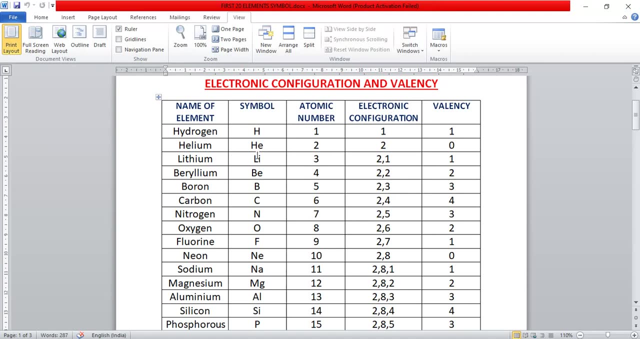 elements. you cannot write the reactions, You cannot write the formula. So you should remember the different, the symbols of different elements with their atomic number. So these two columns you should remember: the symbol and the atomic number. Now let's come to the electronic configuration. Okay, before starting with the electronic configuration, first of all I will 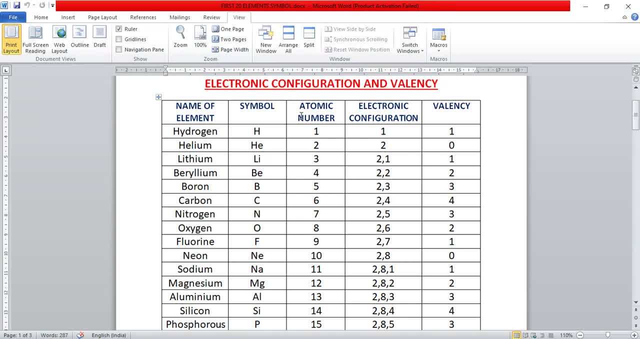 tell you what is atomic number. What is the definition of atomic number? Atomic number is equal to number of electrons or number of protons in an atom. It can be, because in an atom, number of electron is always equal to number of protons. The atomic number is equal to number of electrons. 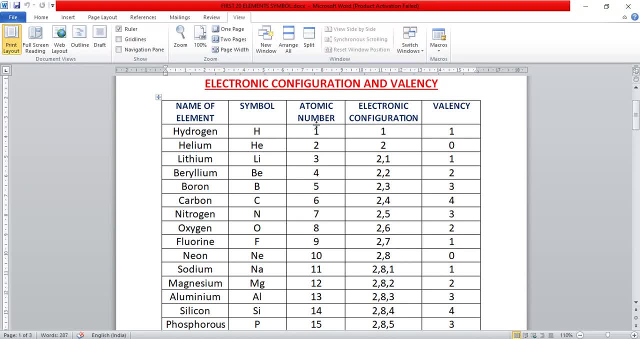 or number of proton, For example hydrogen. it has atomic number one. So how many electrons are present in hydrogen? Only one electron. Likewise, helium has atomic number of two. So how many electrons are present in this helium? Two electrons, Like carbon. Carbon has atomic number of six, So 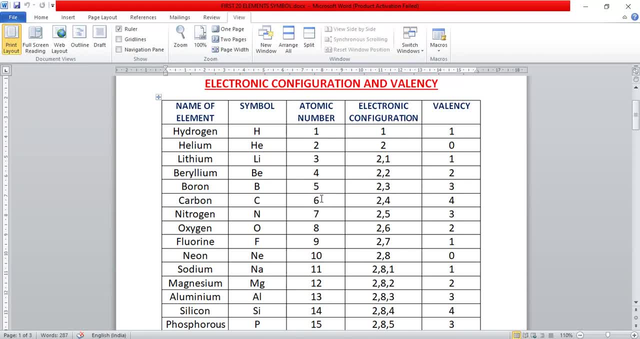 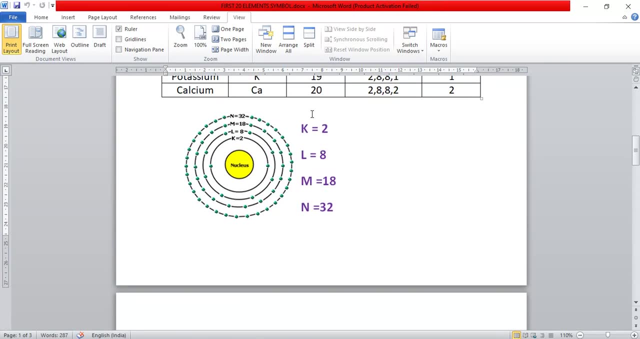 how many electrons are present in this carbon? Six electrons as well as six protons. Okay, and number of protons? Likewise, we have atomic masses also, which is equal to number of neutrons in an atom. Okay, now let's have a look at this diagram. This is a structure of an atom. Okay, in the center. 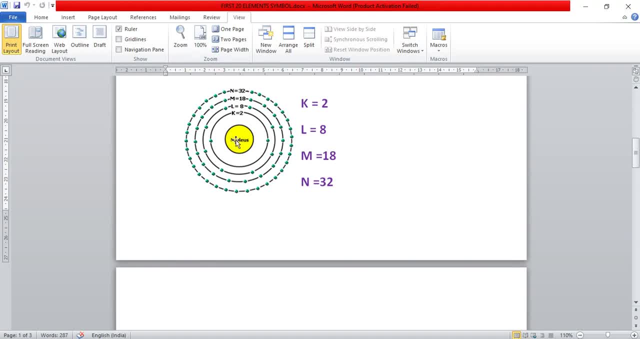 we have nucleus Inside the nucleus. what is present inside the nucleus? Protons and neutrons. Proton has a positive charge and neutron has no charge means neutral charge. So the charge of the nucleus is positive because of the charge of protons. 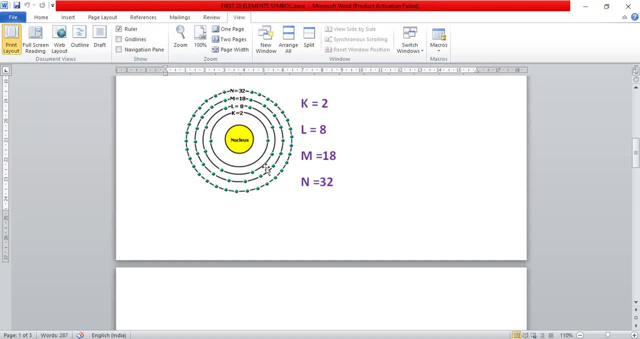 Outside the nucleus, orbits or shells are present in which nucleus revolve around the in which electrons revolve around the nucleus. So these are the different shells in which electrons revolve around. First shell is known as first shell is known as the K shell. First shell is the K shell. 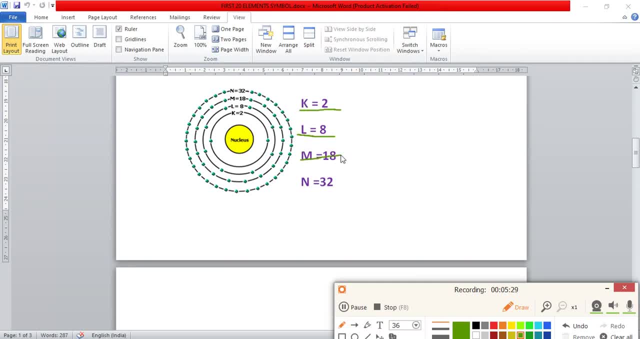 Second shell is L shell, Fourth one is M shell and third one is M shell and the fourth one is the N shell. So K, L, M, N, N. In the first shell, that is K shell, how many electrons can be present? 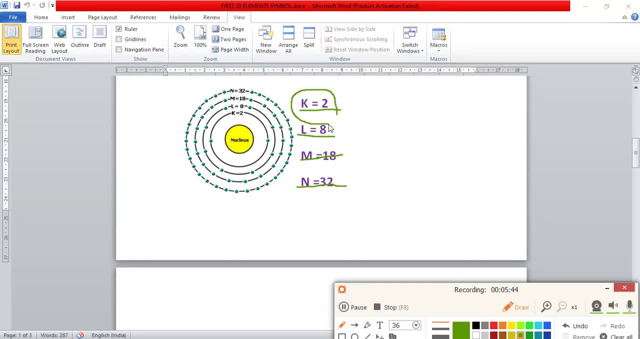 Only two electrons. Only two electrons can be present in this K shell. In the second shell, that is L shell, how many electrons can be present? Only eight electrons. And in the third shell, that is in the M shell, how many electrons can be present? Eighteen electrons. And in the fourth, 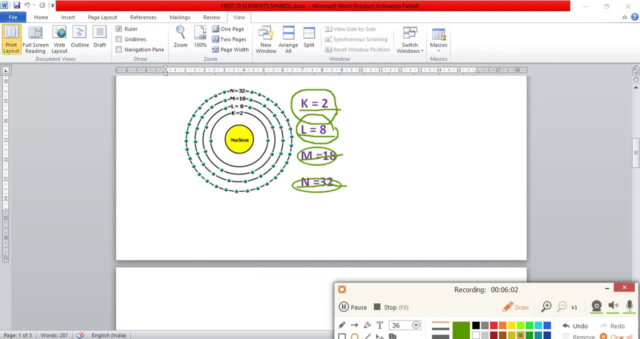 shell. how many electrons can be present? Thirty two electrons. Okay, so these are the distribution of electrons in different shells. In the K shell, only two electrons can be present. In the L shell, only eight electrons. In the M shell eighteen electrons and in the N shell, thirty two. 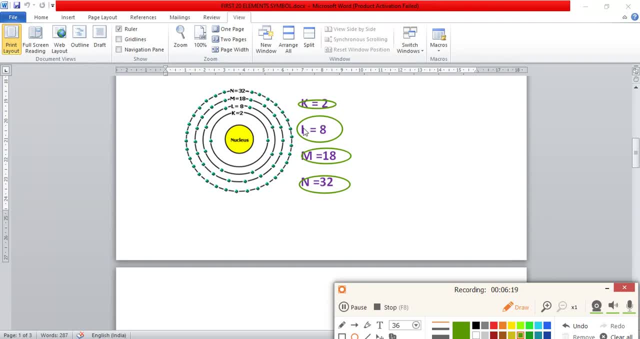 electrons. You should remember that in the first shell, two electrons. second shell, eighteen electrons. third shell: sorry, in the first shell, two electrons. second shell, eight electrons. third shell, eighteen electrons and the fourth shell, thirty two electrons. These are the distribution of electrons in different shells. 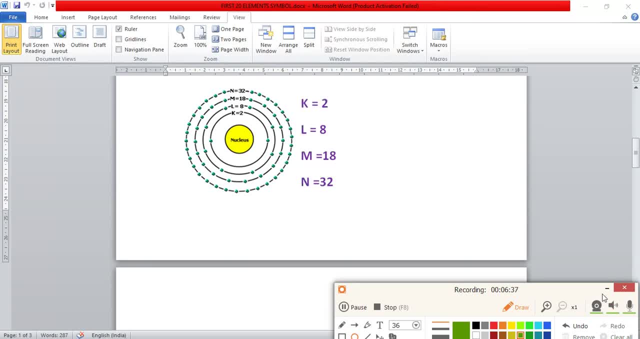 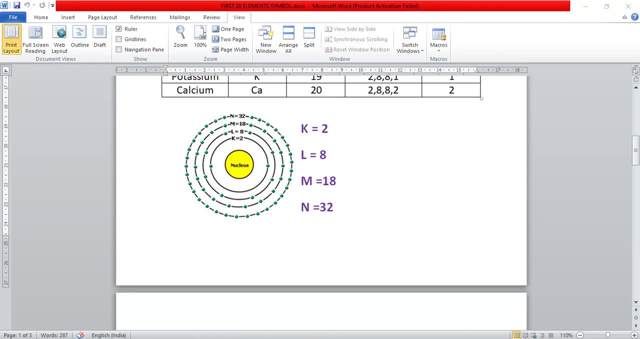 Now we will discuss about the electronic configuration of different elements. So for writing the electronic configuration, what we have to do, We have to make, we have to do like this: K, L, M and N. Suppose we will take the element carbon, Okay, so what is the atomic number? 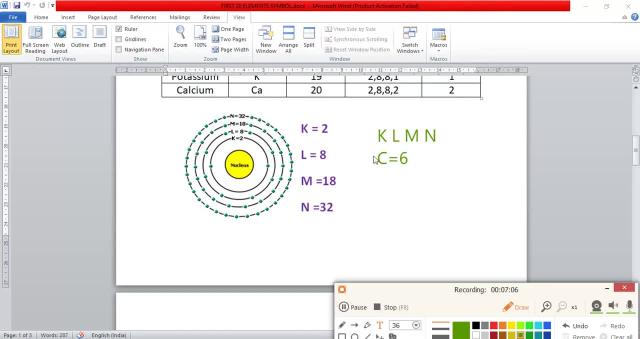 of carbon 6.. So how many electrons are present in this carbon 6,, 6 electrons. So we have to distribute the 6 electrons in the 4 shell. So how we will distribute this 4 electrons. Okay, see in the K shell how many electrons can be, can be accommodated Only two electrons Now. 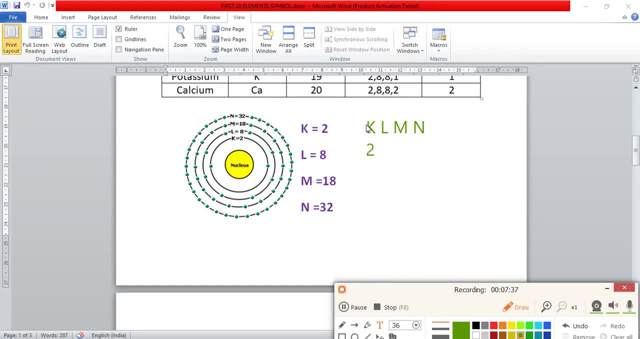 electrons. So from the 6 electrons, 2 electrons we have filled in the K shell. How many electrons are remaining? 6 minus 2 means 4 electrons, So 4 electrons are present in the L shell. Okay, So like this we can write the electron configuration of carbon: Carbon has the atomic 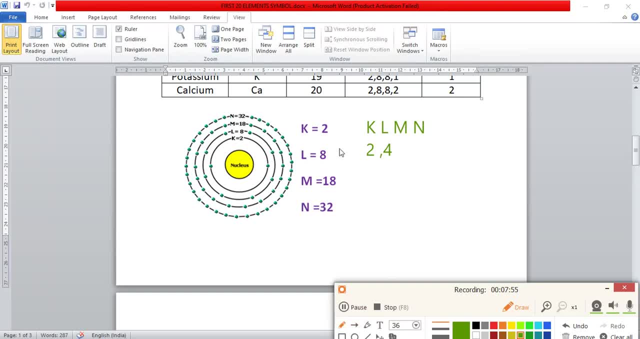 number of carbon has atomic number 6.. Okay, Carbon has atomic number of 6.. 2 electrons can be present in K shell and 6 minus 2 means remaining 4 electrons are filled in the L shell. Okay, Likewise we will see for magnesium, Okay. 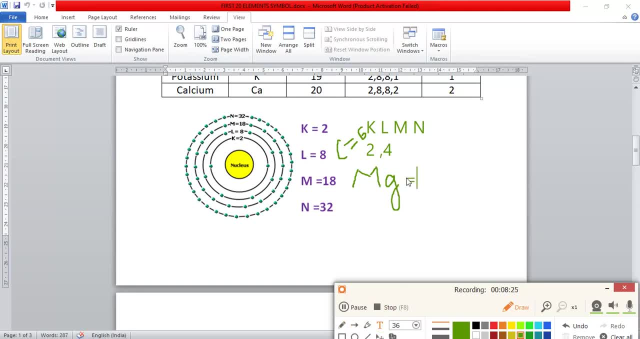 Okay, Magnesium has atomic number of 12.. Now we will represent electronic configuration of magnesium. In the first shell: always 2 electrons. means in the K shell, always 2 electrons. L shell: how many electrons can be present? 8 electrons. We will fill 8 electrons, 8 plus 2, 10 electrons. 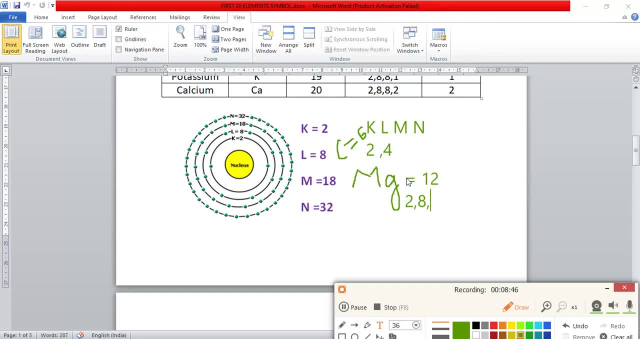 12 minus 10.. How many electrons are remaining? 2 electrons. So we will fill these 2 electrons in the next shell. So this is the electronic configuration of magnesium. Okay, In the first shell, 2 electrons. Next, in the L shell, how many electrons can be filled? 8? 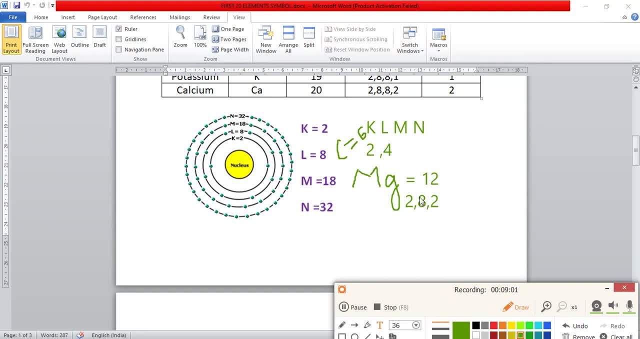 electrons. So 8 electrons we have filled in the L shell, and 8 plus 2 is 10.. So 12 minus 10, only 2 electrons are left. So these 2 electrons will be filled in the M shell, Okay. 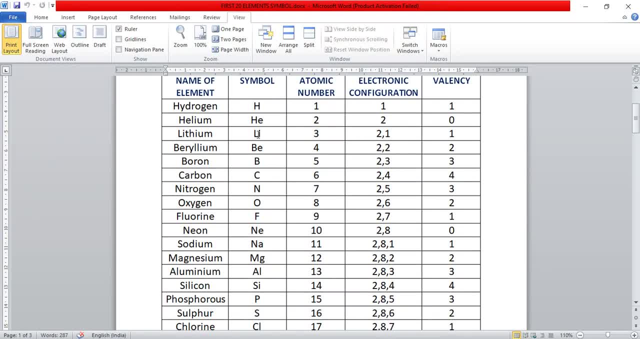 Now we will see the electronic configuration of different elements. Hydrogen: it has atomic number of 1.. So only 1 electron Can be filled in this hydrogen. Only 1 electron is present in this hydrogen. So electronic configuration of hydrogen is 1.. Okay. Next helium. Helium has atomic number of 2.. So 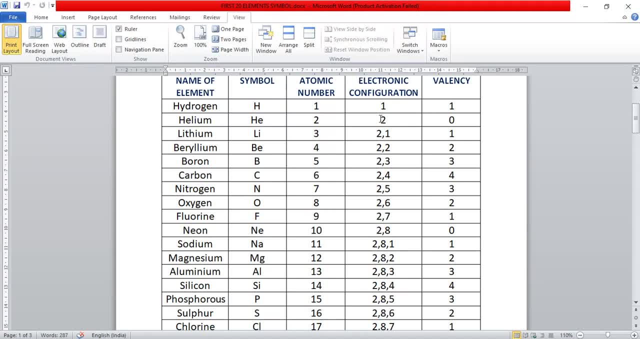 only 2 electrons are present. So electronic configuration of helium can be written as 2.. Lithium has atomic number of 3.. Okay, So in the first shell how many electrons are present? 2 electrons. 3 minus 2 is 1.. So in the L shell, how many electrons will be present? Only 1. 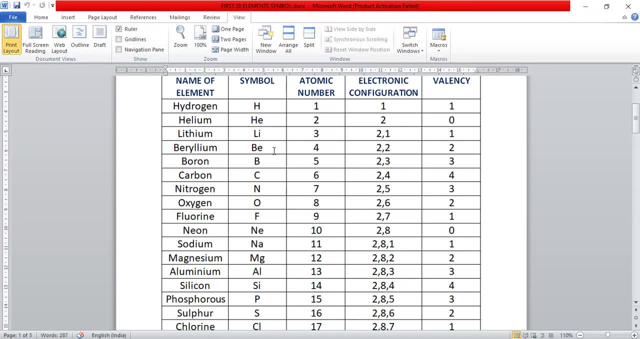 electron. So this is electronic configuration of lithium. So only 1 electron. So only 1 electron, 2 and 1.. Next element is beryllium, with atomic number of 4.. We will write the electronic configuration of beryllium as 2, 2.. Because 2 in the K shell, remaining only 2 electrons. 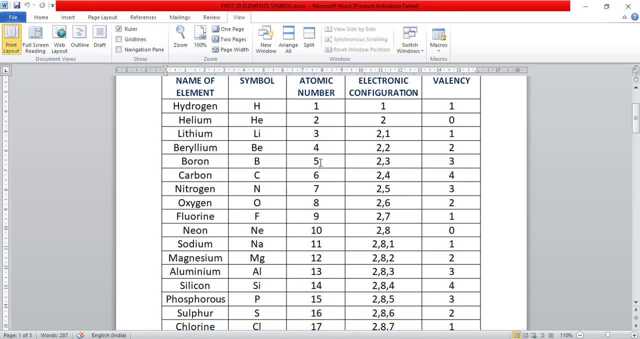 So 2 electrons will be present in the L shell. Boron has atomic number of 5.. 2 electrons in the K shell and in the L shell. how many electrons? 3 electrons. Carbon atomic number: 6. 2 electrons. 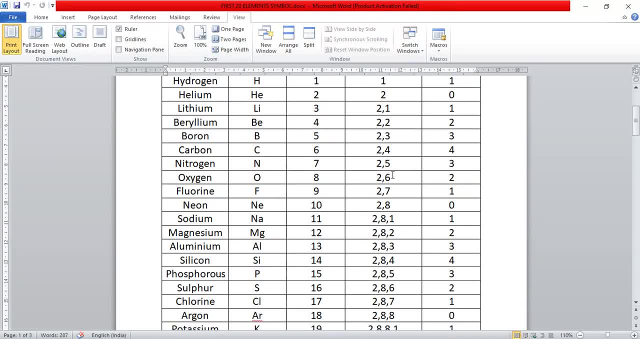 in the K shell, 6 minus 2 is 4.. In the L shell, how many electrons will be present? 4 electrons. Next one is nitrogen, with atomic number of 7.. 2 electrons in the K shell: 7 minus 2 is 5.. 5 electrons will be present in the L shell. 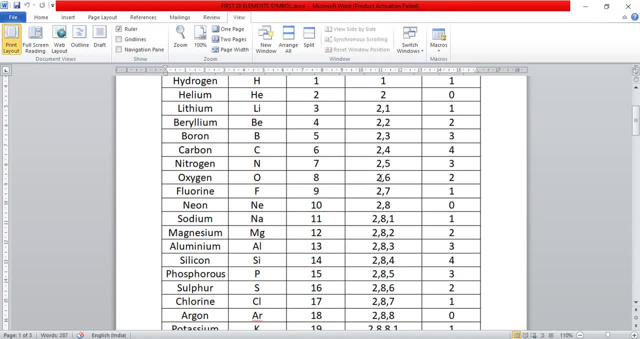 Next one is oxygen, with atomic number of 8.. 2 electrons will be present in the K shell, And 8 minus 2. 6 electrons will be present in the L shell. Next one is fluorine, with atomic number 9.. 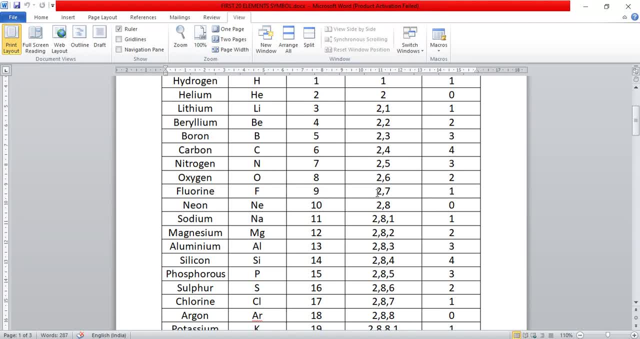 This 9 electrons, how many will be present? 2 electrons. in the K shell, 9 minus 2 is 7.. So in the next shell, how many electrons will be present? Only 7 electrons: Neon, with atomic number. 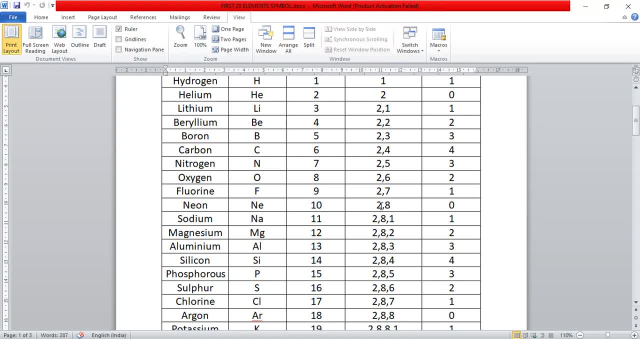 10.. 10 electrons are present in the K shell. So in the next shell, how many electrons will be present in neon? We will write 2 in the K shell. 10 minus 2 is 8.. 8 electrons will be present in. 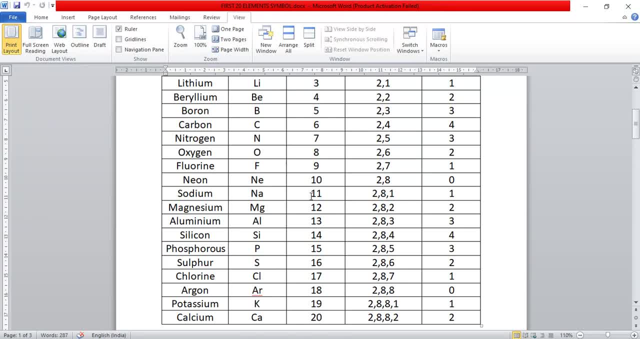 the L shell Sodium with atomic number 11.. This will be present as 2, 8, 1.. 2 in the K shell, 8 in the L shell and 1 electron in the M shell, because we know that in the L shell 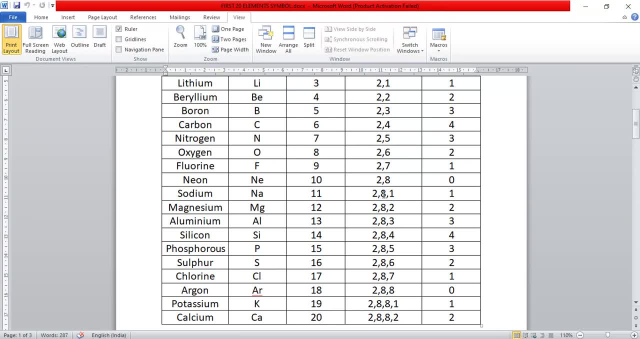 only 8 electrons can be present, Not more than that. So only 8 electrons can be present in the L shell and after that 1 electron we have to give to the m shell. so the electronic configuration of sodium is 2, 8 and 1. next one is magnesium. 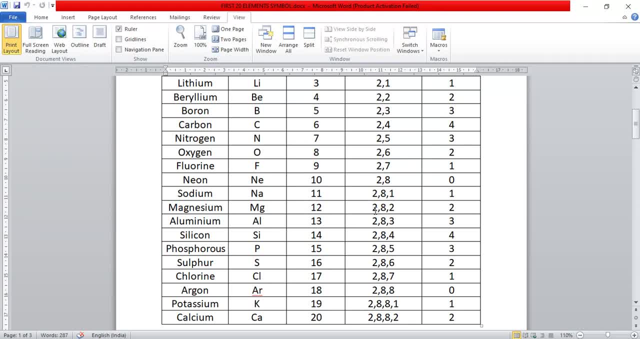 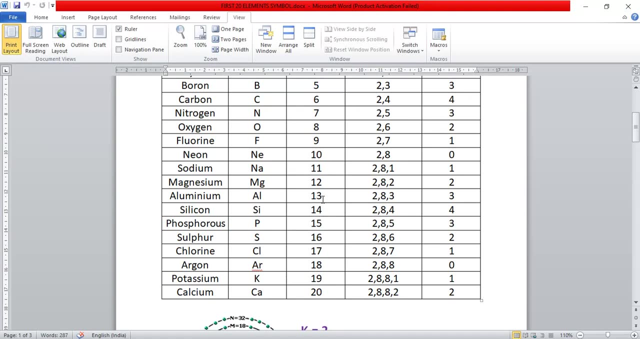 atomic number of magnesium is 12: 2 electrons in the k shell, in the h, in the l shell. how many electrons? only 8 electrons. 8 plus 2 is 10. how many electrons are remaining? 2 electrons- 2 electrons are present in the m shell. likewise for aluminium. atomic number of aluminium is 13, 2 electrons in 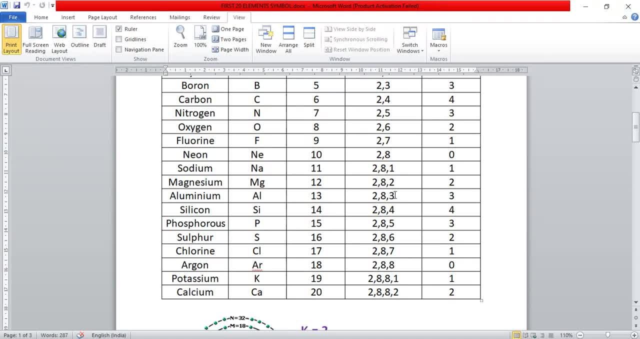 the k shell. in the l shell, 8 electrons and remaining 3 electrons will be present in the m shell. next one is silicon, with atomic number of 14. 2 electrons are present in the k shell. in the l shell how many electrons? 8 electrons and in the m shell remaining 4 electrons. 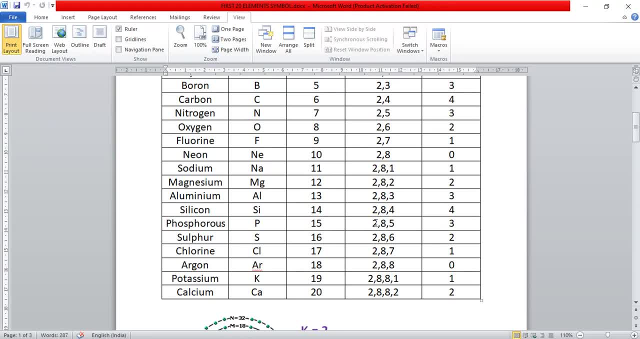 phosphorus with atomic number 15: 2 electrons in the k shell, 8 electrons in the l shell and 5 electrons in the m shell. sulfur with atomic number 16: 2 electrons in the k shell, in the a8 electrons in the l shell and the next 6 electrons will be present in the m shell. 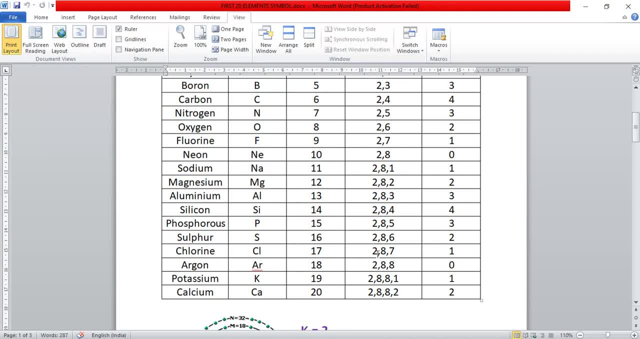 chlorine with the atomic number 17 has a tom. 17 will represent this. 17 electrons has 287 because 2 electrons can be present in the k shell in the next year. only 8 electrons can be present in the next year means that is klm shell. how many electrons can present? 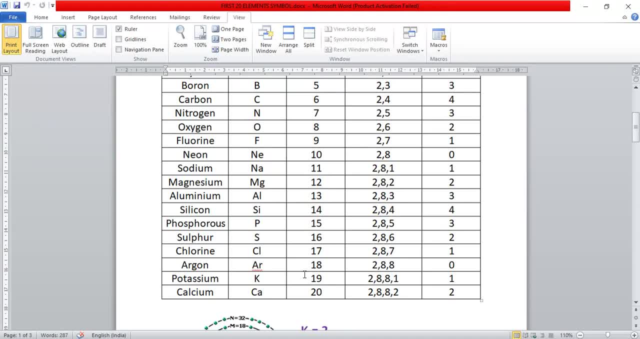 7 electrons we have given to m shell argon with atomic number 18, 2 electrons in the k shell. 18 just represents problem at k shall. so that means there we have to start from trásiter s in. so in simple language it means: and the time we start drawing these узh vegetable. are, we suppose, to consultants? eldritch one thing and the other a euro livrob, dare i will not start on caramel and as you observe, we will add us on in weeks. it then we float in this transaction box and here is our. 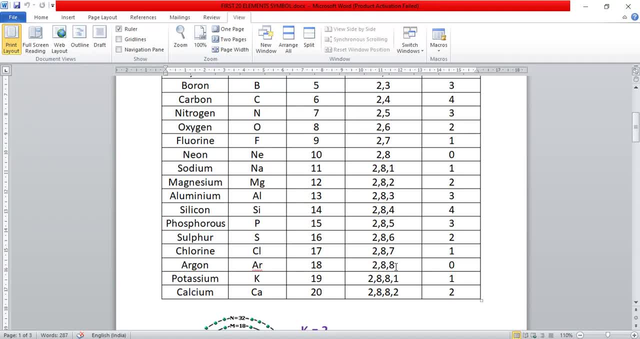 because of hydrogen, with atomic number e, one by y, one by seven, and so we have given to the k shell, in the l shell, 8 electrons and in the m shell also 8 electrons. potassium with atomic number 19, 2 electrons in the k shell, 8 electrons in the l shell, m, in the m shell, 8 electrons again. 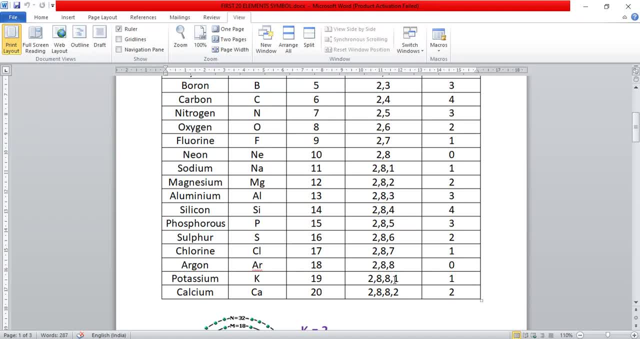 k, l, m and in the n shell. how many electrons? 1 electron. see here we have given only 8 electrons. why? because this is the stable. stay in this. if any atom has 8 electron in its shell, then it will become stable. so we have given 8 electron in the k- l, m shell and 1 electron we have given to. 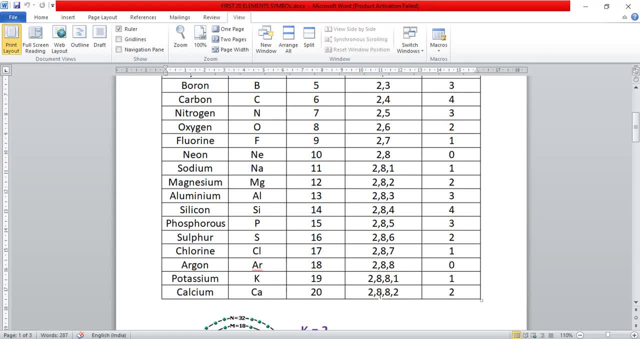 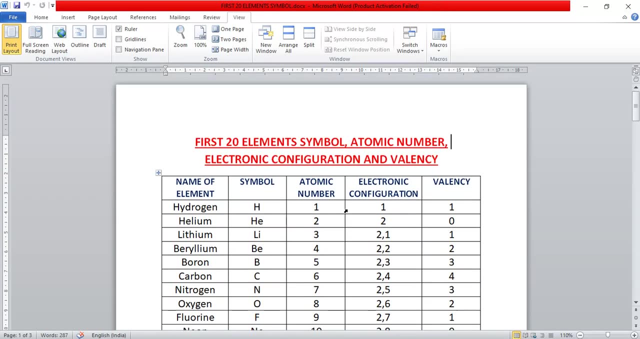 n shell: okay. likewise for calcium: 2, 8, 8, 2 k shell: 2 electrons. l shell: 8 electrons. m shell: also 8 electrons. and in the n shell how many electrons are present? 2 electrons, okay. so like this, we have to write the electronic configuration of the elements we have to, to remember that in the k. 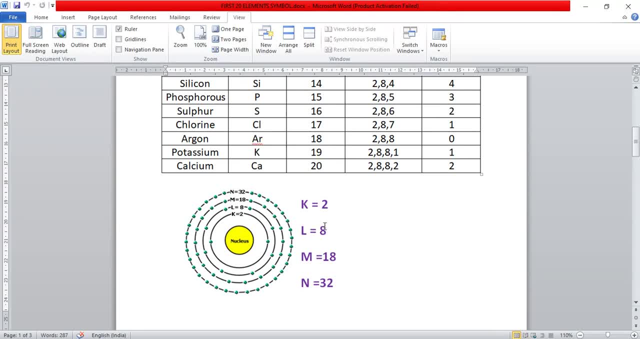 shell, always 2 electrons. we have to fill in the l shell: always 8, not more than that. and then we have to write the electronic configuration of the elements. we have to write the electronic configuration of the elements. we have to fill in the l shell and in the n shell. 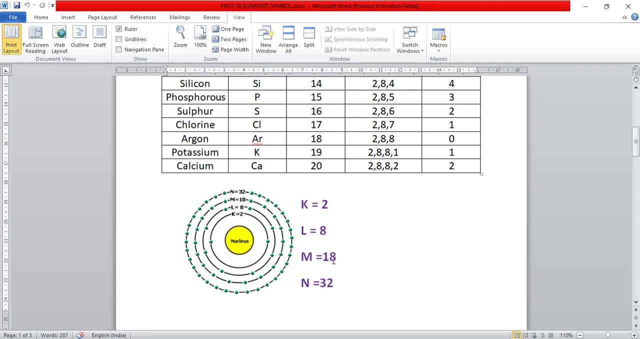 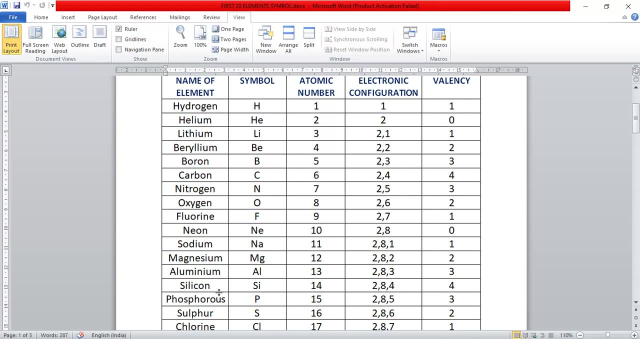 next electrons will go into the m shell, that is, it can accommodate 18 electrons and the n shell can accommodate 30, 32 electrons. now we'll see how to write the valency. valency is the combining capacity of an atom. okay, the definition of valency is combining capacity of an atom, so different. 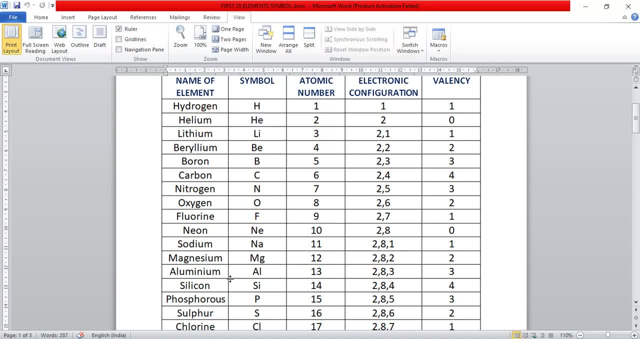 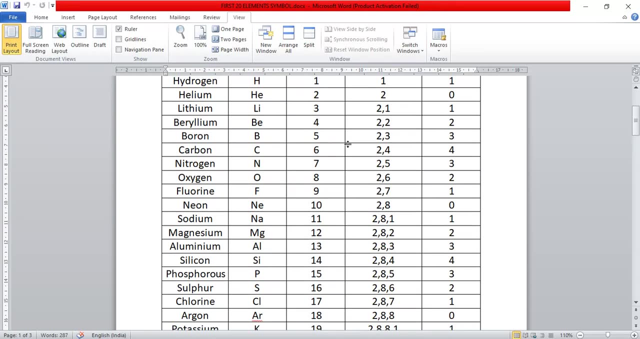 elements have different types of valencies. for example, a particular group also has a fixed valency. group 1 has different valency. group 2 will have different valency. noble gases- group number 15, okay, or inert gases. noble gases are also known as inert gases. they will have valency equal to. 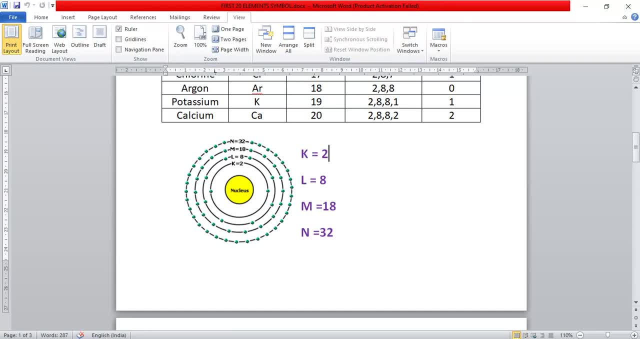 zero. okay, why the noble gases have valencies equal to zero? noble gases have zero valency. noble gases have zero valency. why does noble gases have zero valency? okay, we all know that noble gases, or the inert gases, they don't, they will. they're, they're non-reactive. okay, they will not react with any other elements or atoms, because they. 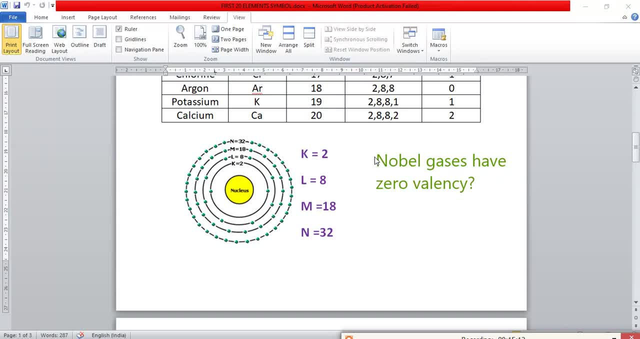 are stable in their state means their outer shell is completely filled. either they are duplet or or either they have a duplet or a octet. structure means in the outer motion, either they have two electrons or they have eight electrons in their outer motion. okay, they have. 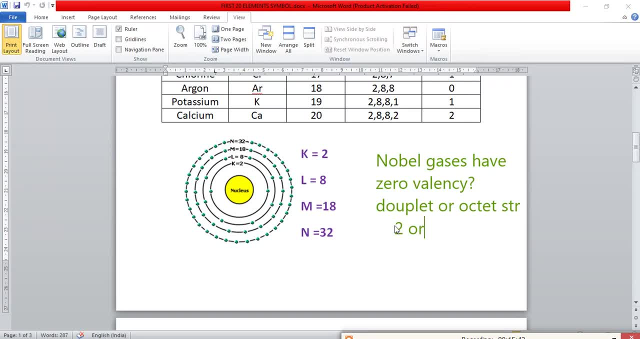 uh two or eight electrons in their outer motion in their outermost shell. If the noble gases have two or eight electrons in the outermost shell, it means they are stable. They have a duplet or an octet structure. They don't want to gain. 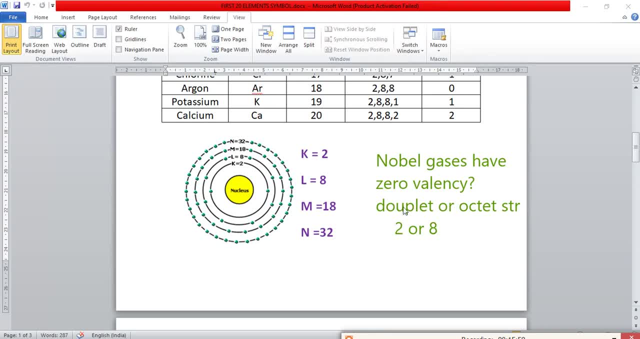 electron, nor they want to lose electron, So they have a valency equal to zero. So why noble gases have zero valencies? Because they are stable. They have a duplet or an octet structure. It means they don't want to gain or lose electron, So their valency is always equal to zero. Okay. 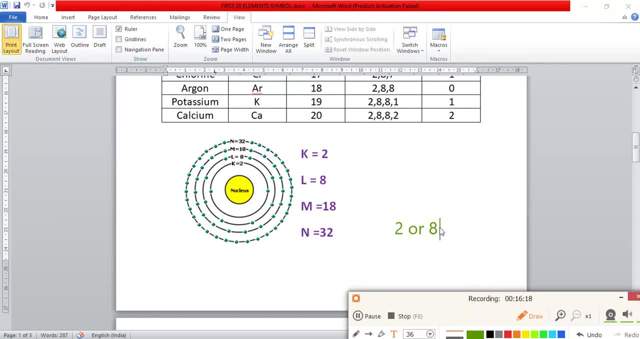 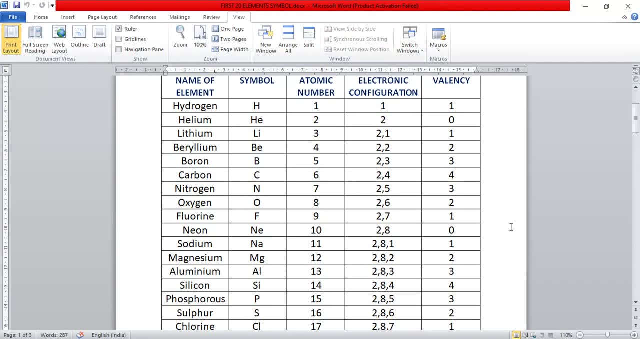 Okay, Now we'll see how we have to write the valency For hydrogen. what is the atomic number of hydrogen? One? Electronic configuration: one. How many electrons are present in hydrogen in the outermost shell? One, So one is the valency of hydrogen For helium? only two electrons in 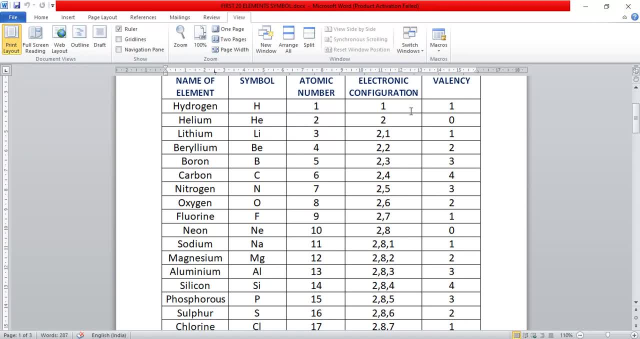 the outermost shell. But we know helium is a noble gas. It has two electrons in its outermost shell, means it is stable in its state. So its valency is equal to zero. Helium has a valency which is equal to zero. All the noble gases like helium, neon, argon, krypton, they have a valency. 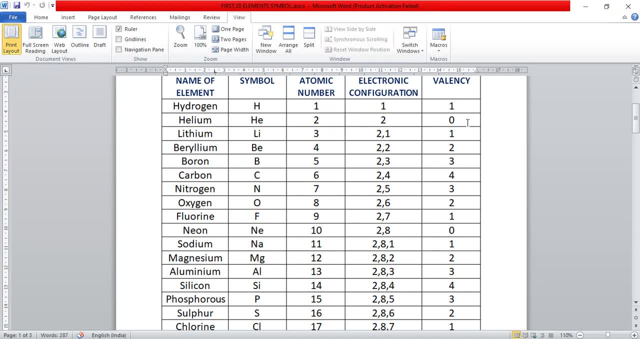 equal to zero. because they are stable in their state. They don't need to gain or lose electrons. Next one is lithium at atomic number three. So how we will write the electronic configuration of lithium Two and one. How many electrons are present in the outermost shell of lithium One? 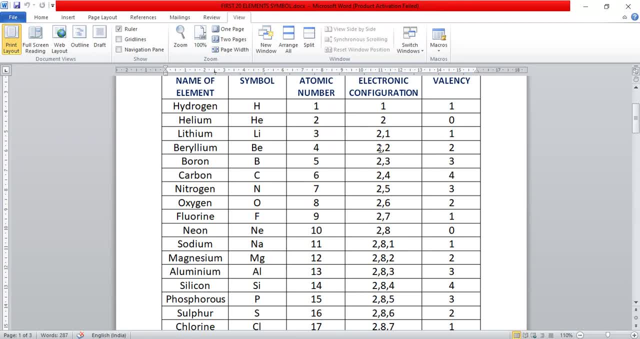 electron. The valency of lithium is one. Next one is beryllium. Two comma two Means two electrons are present in the outermost shell of beryllium, So valency of beryllium is two. Next one is boron. Boron has atomic number of five. 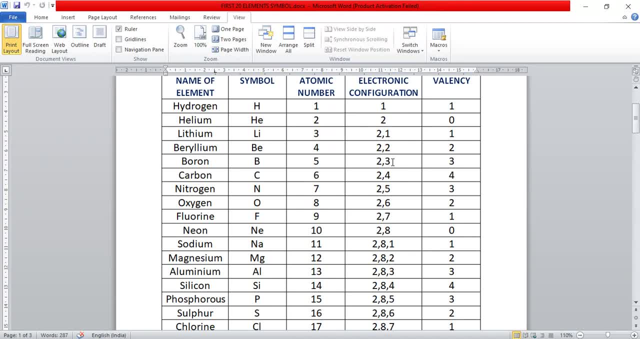 Electronic configuration: two, three. Three electrons are present in the outermost shell, So the valency of boron is three. Next one is carbon, with atomic number six. Electronic configuration is two, four, And the four electrons are present in the outermost shell, So the valency 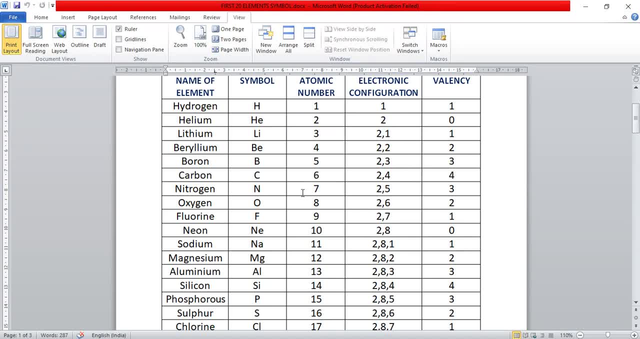 of carbon is four. Next one is nitrogen. Now we have to see- Okay, So nitrogen has an atomic number of seven- How we will write the electronic configuration: Two, five. It will not donate this five electron because for donating this five electron, it needs large amount of energy. So what it will do To complete its 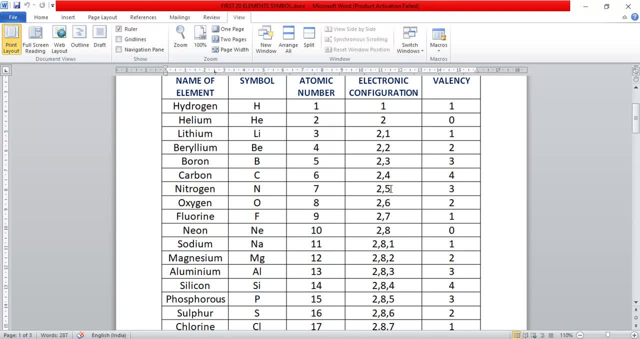 octet means to fulfill its shell or to become stable. What it will do? It will take three electrons from somewhere. If it will take three electrons, then how many electrons it will have in the outermost shell? Five plus three, eight electrons. 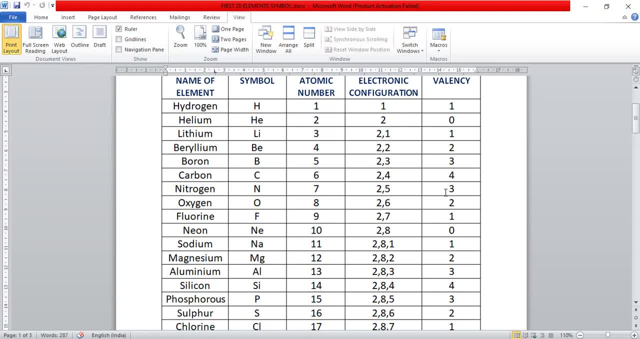 Okay, So the nitrogen has a valency of three. Next one is oxygen. Oxygen is atomic number of eight, Two, six. For fulfilling its shell to become octet structure, how many electron it needs. Six plus two means eight. Six plus two means two electron it needs to complete its octet. 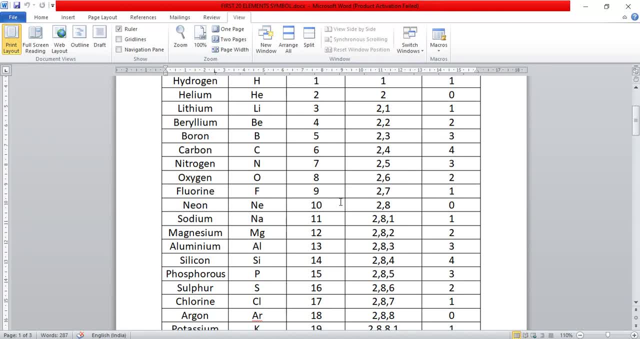 So the valency of oxygen is two. Next one is fluorine. Atomic number nine, Two, seven. How many electron it needs to complete its octet. Six plus two means eight. So the valency of fluorine is one. Next one is, again, our neon. 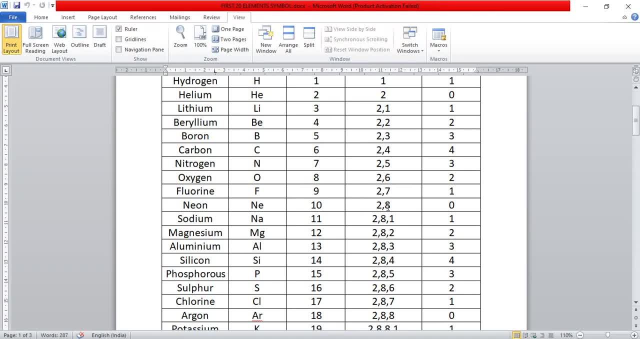 Neon is a noble gas. It has already eight electron in the outermost shell, So it don't need to gain or lose electron. So the valency of neon is zero. Next one is sodium: Two eight one, One electron in the outermost shell. So the valency of sodium is one Magnesium- atomic number 12.. Two eight. 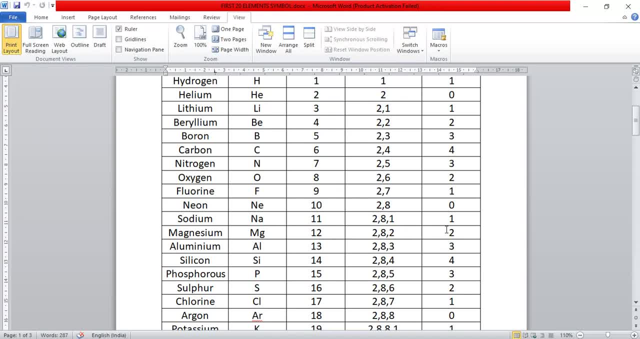 two. Two electrons in the outermost shell. So the magnesium has a valency of two. Next one is aluminium. Two, eight, three In the outermost shell. how many electrons are present? Three electrons, So the valency of aluminium is three. Silicon has atomic number 14.. So the 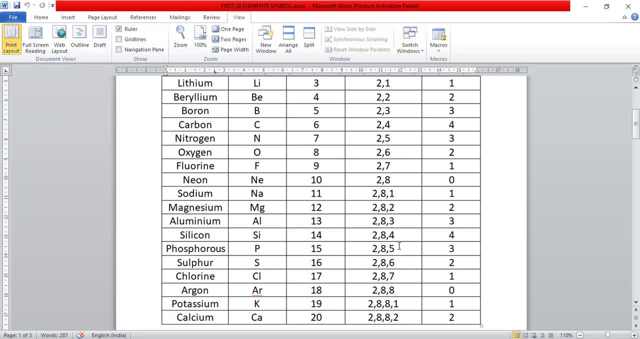 electronic configuration of silicon is two eight, four. So the valency of silicon is four. Okay, it can donate to its four electrons. So the valency of silicon is four. Next one is phosphorus, with atomic number 15.. Electronic configuration: two eight, five. Again, we have five electron in the 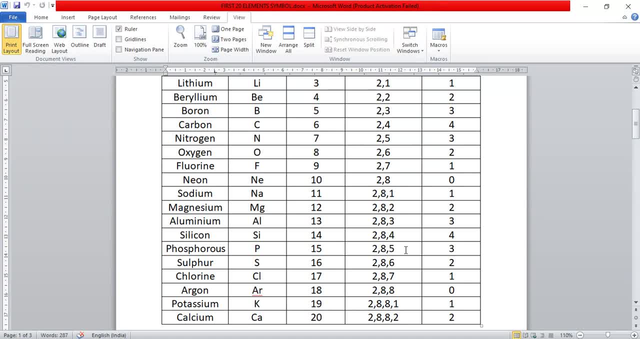 outermost shell. So the valency of silicon is four. Next one is phosphorus, with atomic number 15.. It cannot donate its five electron. What it will do To become stable, it will accept three electrons. Means in the outermost shell it should have eight electrons. So it will become stable. 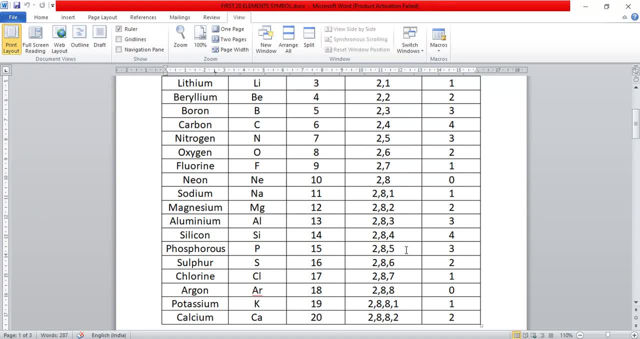 So what it will do? It will accept three electrons and it will become stable. So the valency of phosphorus is three. Eight minus five means three. Next one is sulfur, 16.. Atomic number: 16.. Electronic configuration: two, eight, six, Eight minus six. Only two electron is need to become stable, So the 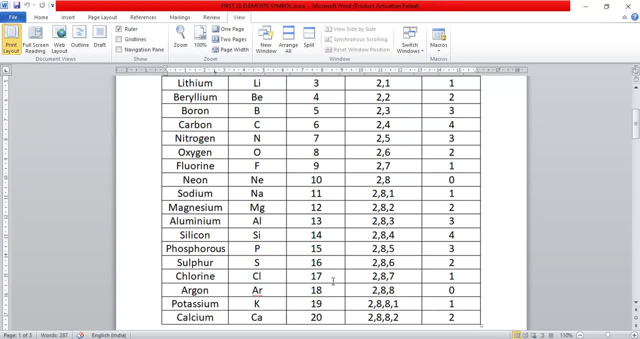 sulfur has a valency of two. Next one is chlorine 17.. Atomic number two: eight seven. How many electron it needs to complete its octet? Only one electron. So the valency of chlorine is one. Next one is argon. Again, it is a noble gas. Now we'll see the electronic configuration of argon with. 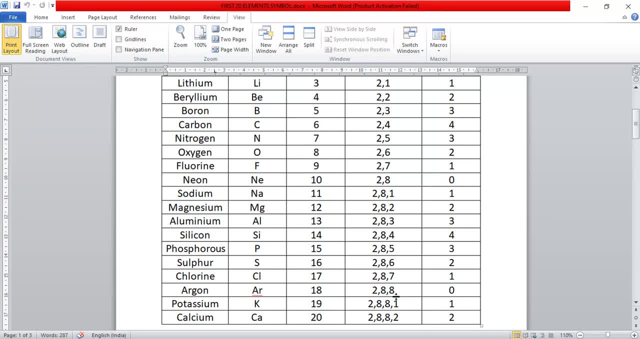 atomic number 18.. Two, eight, eight. It has eight electron in the outermost shell, So it don't need to lose or gain electron. So the valency of argon is zero. Potassium has atomic number 19.. So the 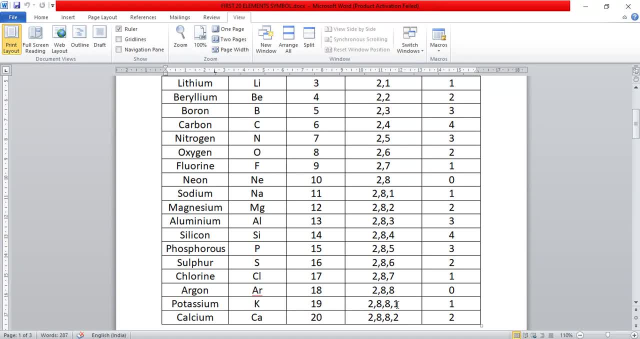 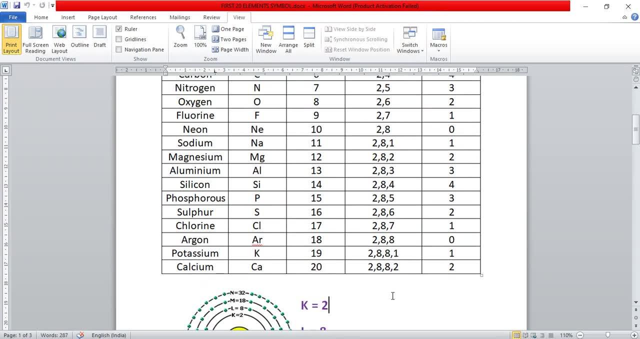 electronic configuration of potassium is two, eight, eight, one, So it has one electron in the outermost shell. So the valency of potassium is one. Next one is calcium with atomic number two. What is the atomic number of calcium? 20.. Now we'll. 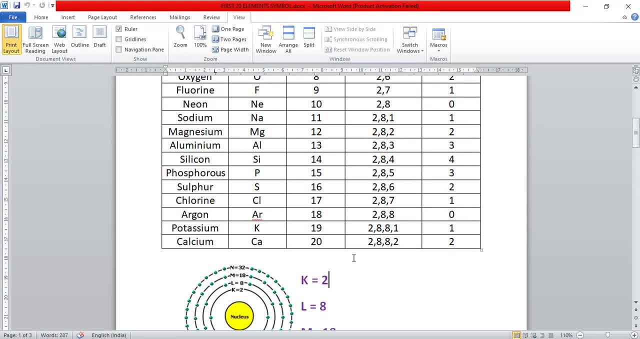 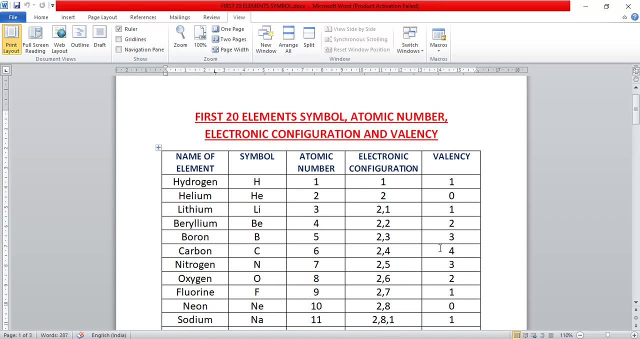 see the electronic configuration of this calcium: Two, eight, eight, two. How many electron it has in the outermost shell? Only two electrons. So these two electrons it can donate to any other calcium. So the atomic number of calcium is two. Okay, Now we have seen how we can find the 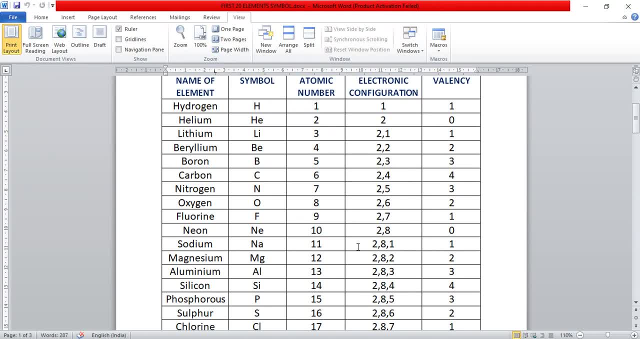 valency of different elements. So now it's, I think it is clear for you how you have to write the atomic number, how you have to write the electronic configuration and the valency For doing so. you have to remember the atomic number. It's very important that you should remember. 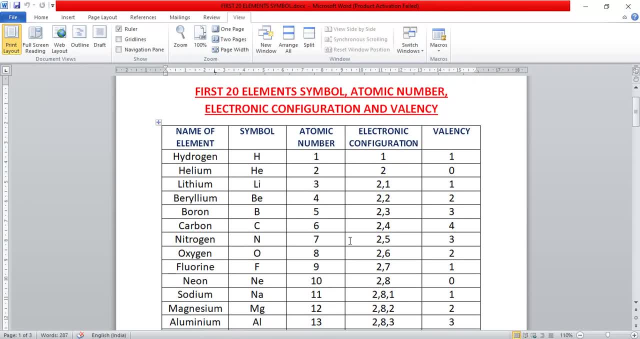 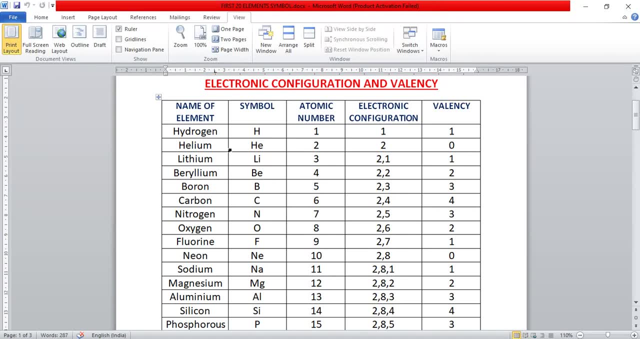 the atomic number from hydrogen to calcium. For eighth, ninth and tenth student, it's very important that you should remember the first 20, first 20 element symbol atomic number so that you can write the electronic configuration and valency and 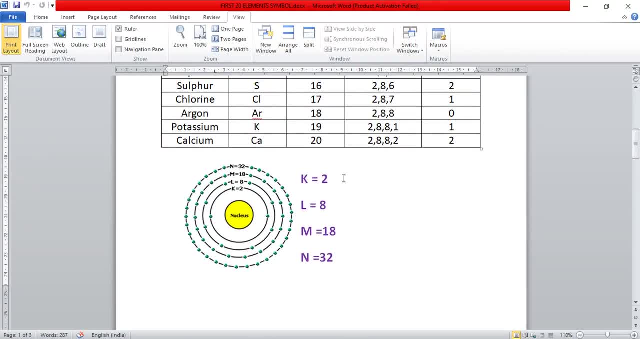 you can write any reaction and formula using these symbols. Okay, Now one more thing I want to tell you: Metals. Okay, Do you know what is the definition of metals? Metals are those elements which can donate electrons. Okay, Donate electrons, donate electrons. Metals are those elements which can donate electrons, Means. 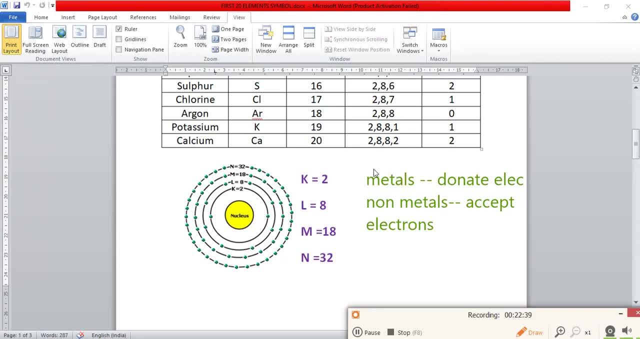 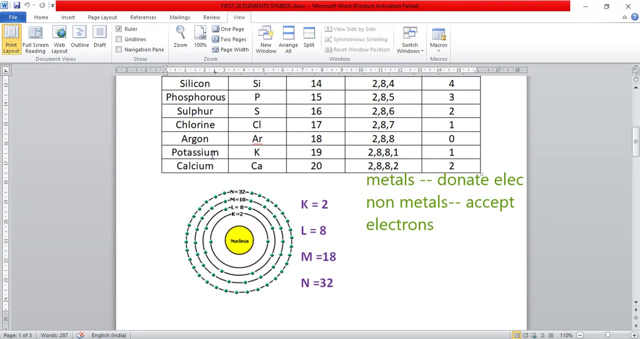 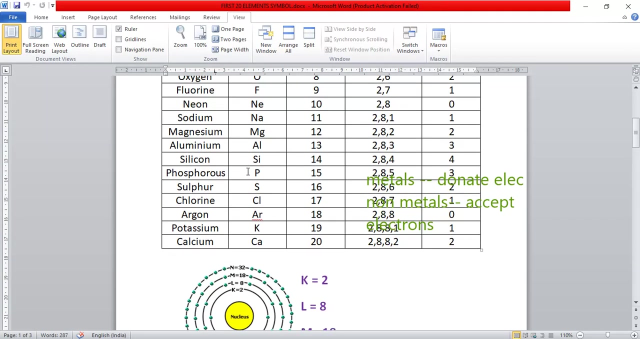 these metals can give their extra electrons to any other element. None metals, they accept the electrons. So from this, from this chart, we can see that potassium, calcium, they can easily donate their outermost electron to some any other element. So these are the metals: calcium, potassium. 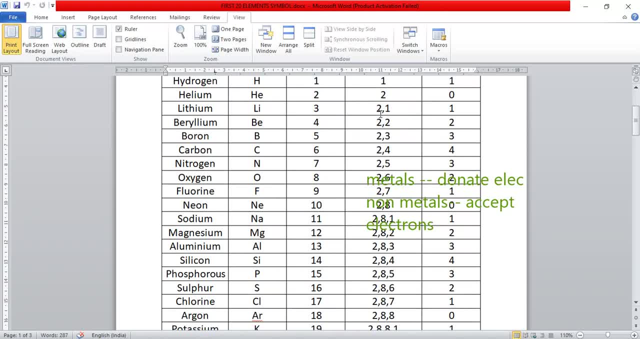 even your this one: lithium, beryllium, boron, carbon the boron- these can donate their electrons to any other element. So these are the metals. Okay, Like go, your suppose we'll take the example of aluminium. 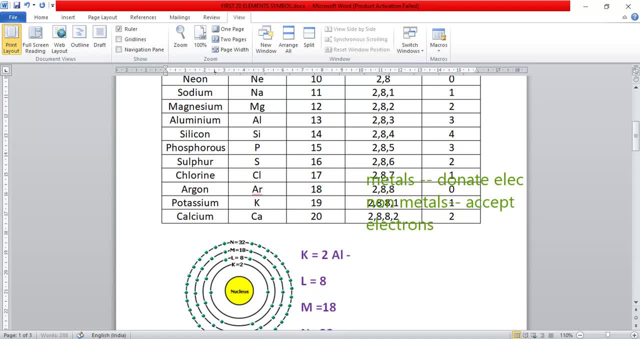 Aluminium has atomic number 13.. We can write the electronic configuration as 2,, 8,, 3.. How many electron it has in the outermost electron? 3 electrons. So it can donate its 3 electron to any other element. So our aluminium is a metal. Okay, Likewise. 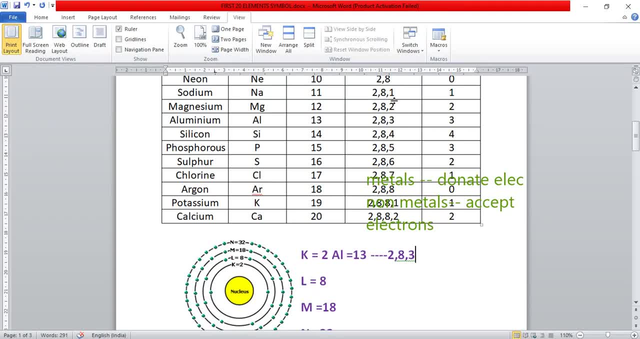 magnesium is also a metal. It can donate its electron. Sodium is also a metal. It can donate its electron. Now we'll see one example of non-metal. Suppose we'll take chlorine. Chlorine has atomic number of 17.. How we'll write the electronic configuration of chlorine? 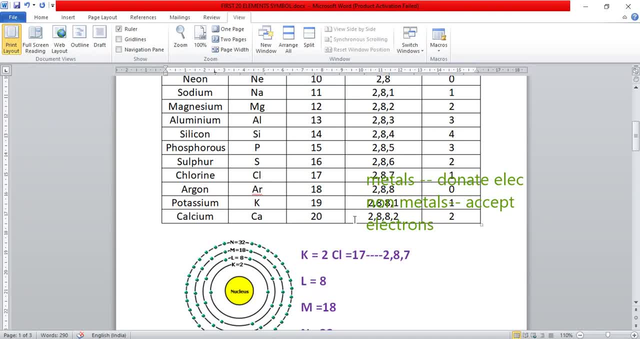 2, 8 comma 7.. So to become stable, to get 8 electron in the outermost shell, what it will do? It will accept one electron. So chlorine is our non-metal. It has a tendency to accept the electron. So 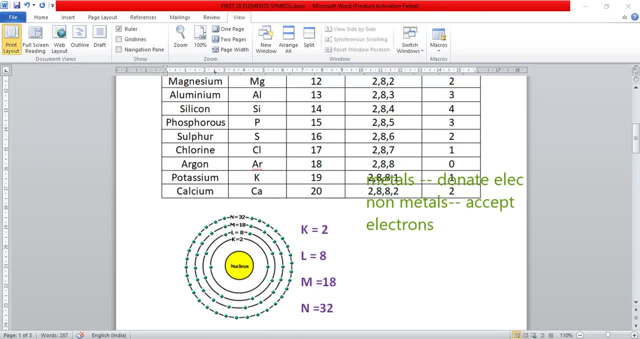 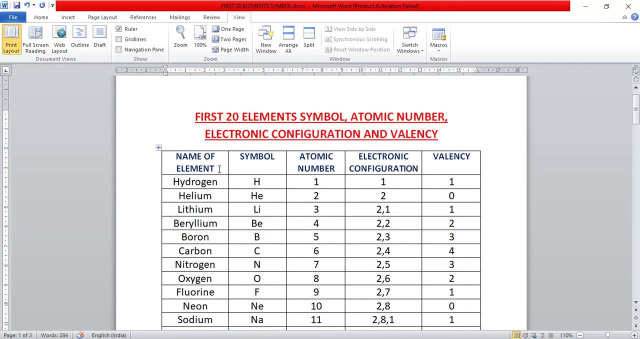 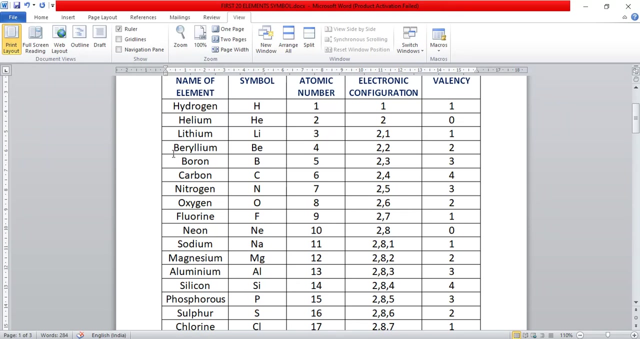 chlorine is our non-metal. So now it's clear. So now it's clear what are metals and what are non-metals. Metals are the elements which can donate their electrons and non-metals are the elements which can accept the electron. So you: 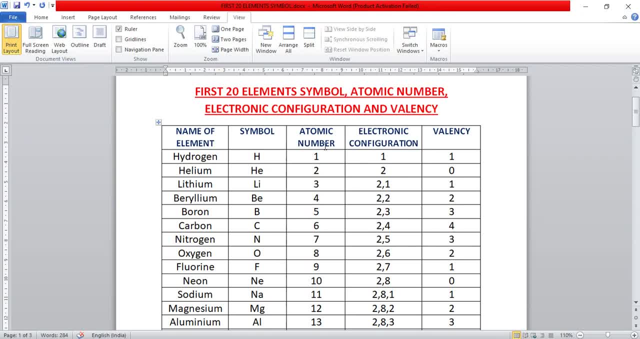 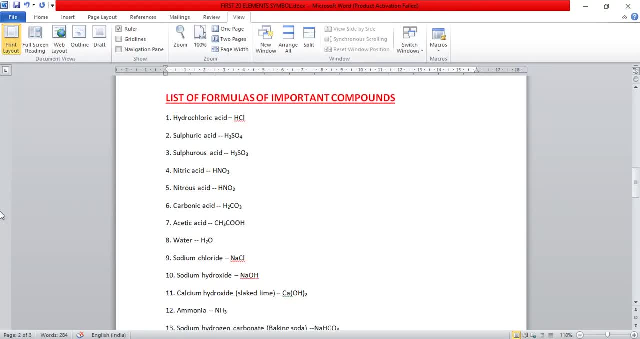 should remember the name of the elements with the symbol, atomic number, electronic configuration and valency. Okay, now let's come to the list of formulas of some important compounds which you should know, Because without knowing the formula of this compound, you cannot write a reaction. 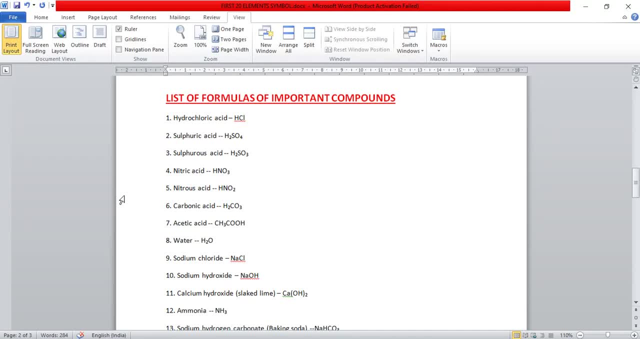 Suppose you will get the formula of the represents of a reactant, So you will get the formula of the. get in your exam, write the reaction between zinc and hydrochloric acid. for writing the reaction you should know the symbol of zinc. so what is the symbol of zinc, Zn, and what is the formula? 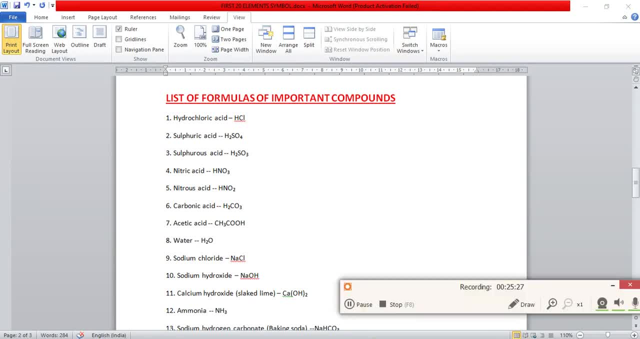 of hydrochloric acid, HCl, so you can easily write the reaction: Zn plus HCl. Zn plus HCl gives ZnCl2, ZnCl2 plus plus H2. okay, if you know the formula of zinc and hydrochloric acid, then only you can write. 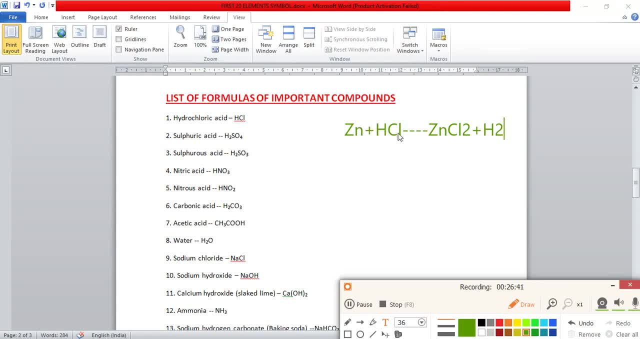 the symbol of zinc: Zn plus HCl. so when zinc will react with hydrochloric acid will get zinc chloride: ZnCl2 plus H2 gas. H2 gas will evolve in this reaction. okay, so for writing the formulas, for writing the reactions and all you should remember the formulas. okay, now let's see the different compound and their 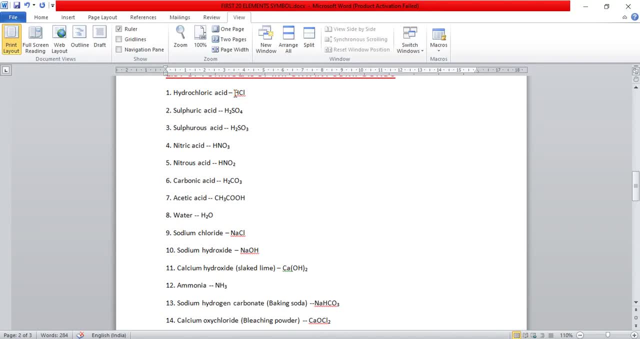 formulas. hydrochloric acid is a very important acid. what is the formula of the hydrochloric acid, HCl? next one is sulfuric acid. the formula of sulfuric acid is H2SO4- sulfuric acid, the. what is the formula of sulfuric acid, H2SO3? the don't get confused between sulfuric acid and sulfuric acid. sulfuric acid has a formula of H2SO4 and sulfuric acid has a formula of H2SO3. next one is nitric acid. what is the formula of nitric acid? HNO3. 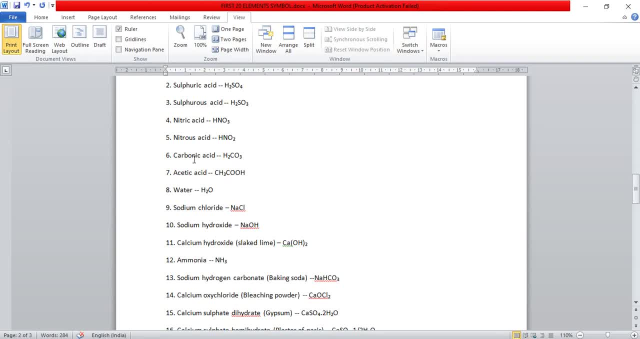 nitrous acid. it has a formula of HNO2 carbonic is. it has a formula of H2CO3 acetic acid. what the formula of HNO3 is? H-ierenic Acid, H 2- CO3, somebody Who Can See This? 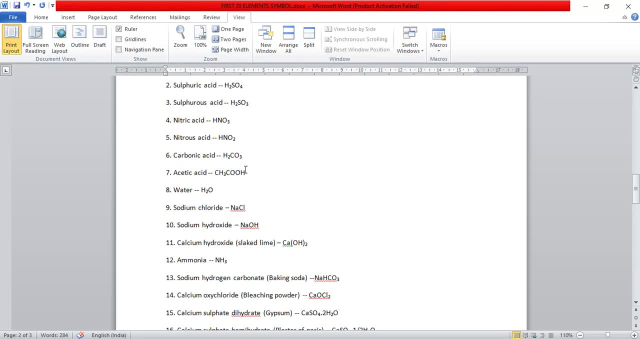 Ok, I'm writing it down: never Thoragoiyanda. Remember that I should say H-ie nochi acid. What is the formula of acetic acid, CH3COOH? Do you know the common name of this acetic acid? What is the common name of acetic acid? Common name of acetic acid is vinegar. Okay, So the 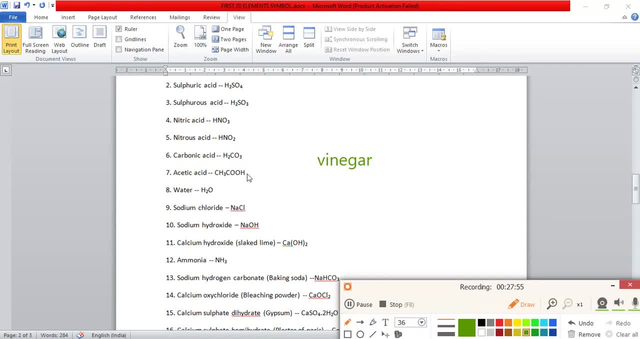 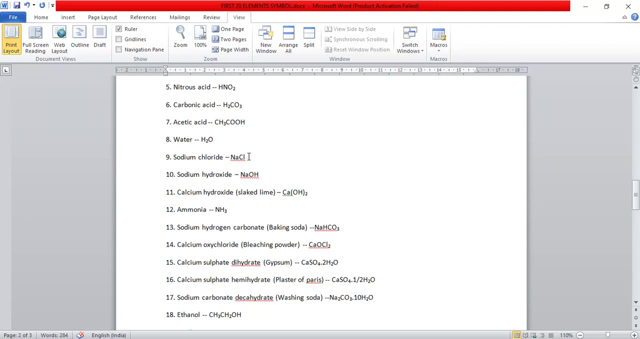 common name of acetic acid is vinegar. Next one is water. What is the formula of water? Water Formula of water is H2O. You all know this formula. Sodium chloride: What is the formula of sodium chloride, NaCl. What is the common name of sodium chloride? Common salt, The salt which 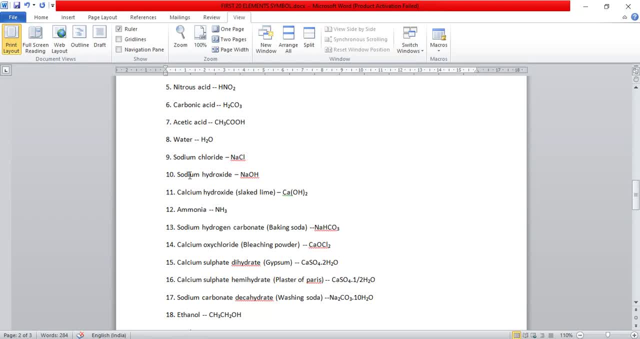 we use in our food is sodium chloride. Next one is sodium hydroxide. The formula of sodium hydroxide is NaOH. Next one is calcium hydroxide. The common name of calcium hydroxide is slate lime. The formula of calcium hydroxide is CaOH- whole 2.. Next one is amylase. Next one is: 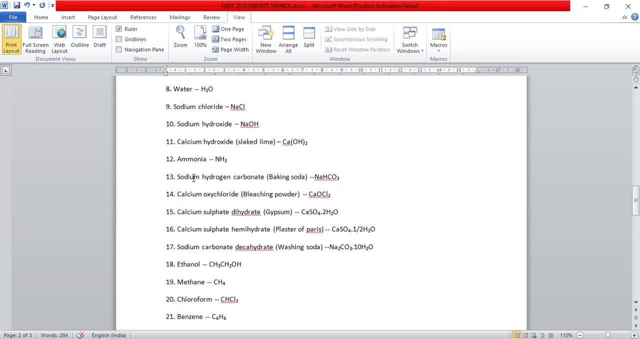 ammonia, with the formula of NH3.. Next one is sodium hydrogen carbonate, Baking soda. Do you know what is the use of baking soda? Yes, It is used in the bakery or for making the cakes and the breads. Okay, It is used to make the cake soft and spongy. The formula of baking soda, or sodium. 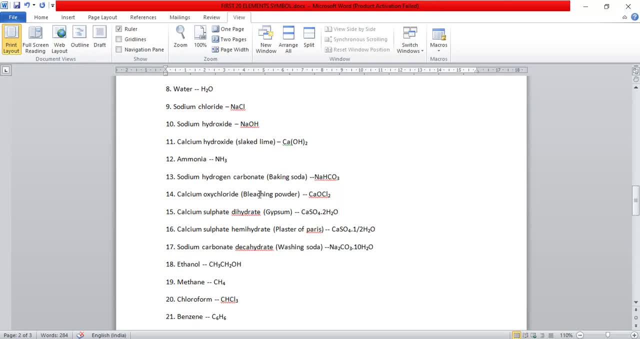 hydrogen carbonate is NaHCO3.. Next one is calcium oxychloride bleaching powder. What is the formula of this bleaching powder? CaOCl2.. The formula of this bleaching powder is CaOCl2.. The formula of this bleaching powder is CaOCl2.. 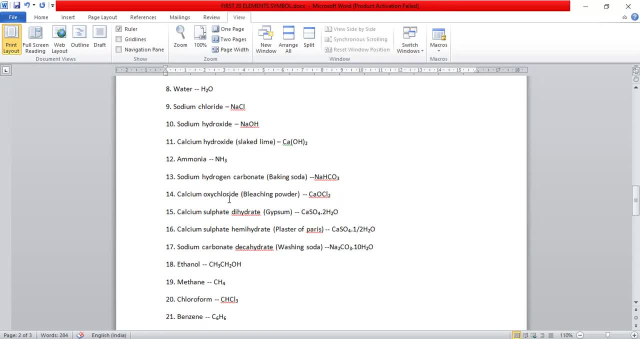 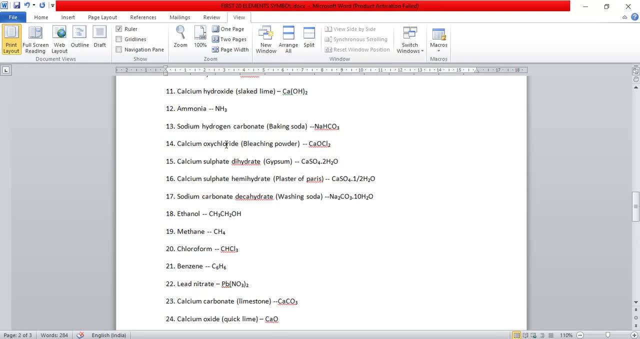 What is the use of this bleaching powder? It is used for killing the germs in the water or it has many other uses also. It is also used for bleaching in paper industry, as a bleaching agent in the paper or the textile industries. Next one is calcium sulfate dihydrate, that is, gypsum, The. 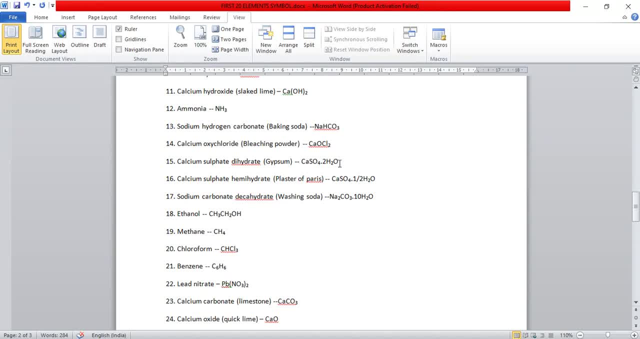 formula of gypsum is CaSO4.2H2O. This 2H2O is attached as a water, as a molecule of water of crystallization means two unit of water of crystallization is attached with this water, This formula. unit of calcium sulfate. Next one is calcium sulfate hemihydrate. Hemi means half. 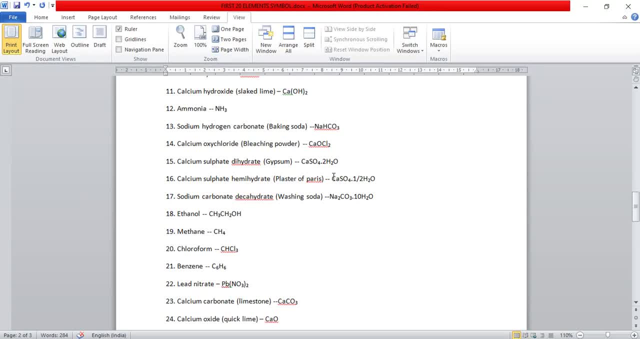 This is known as plaster of Paris. The formula of plaster of Paris is CaSO4.2H2O. Next one is sodium carbonate decahydrate. This is washing soda. Common name is washing soda. The formula of washing soda is Na2CO3.10H2O means 10H2O. water of crystallization is attached with Na2CO3.. Next. 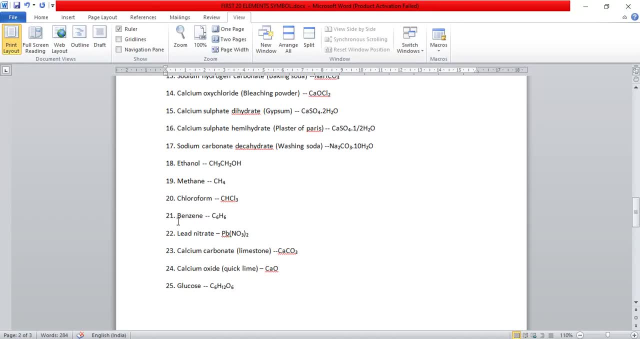 one is ethanol. The formula of Na2CO3.10H2O is attached with Na2CO3.. Next one is ethanol. The formula of ethanol is CH3CH2OH, or you can also write as C2H5OH. Next one is methane. It is one. 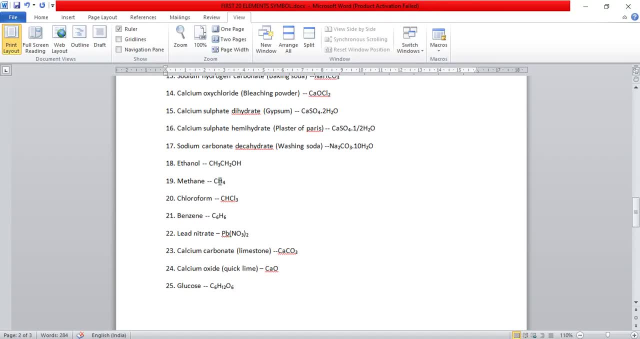 of the most important carbon compound. It has a formula CH4.. It is the main constituent of biogas methane. Next one is chloroform. The formula of chloroform is CHCl3.. Benzene, a 6 carbon compound. 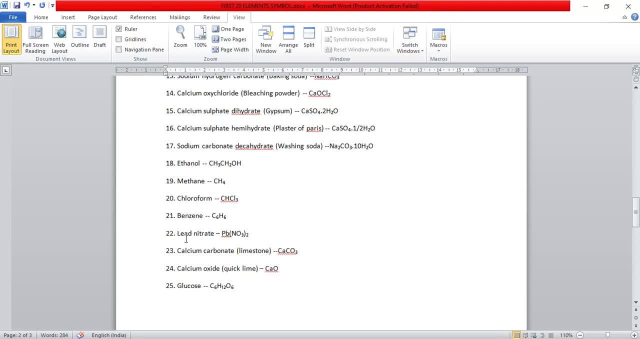 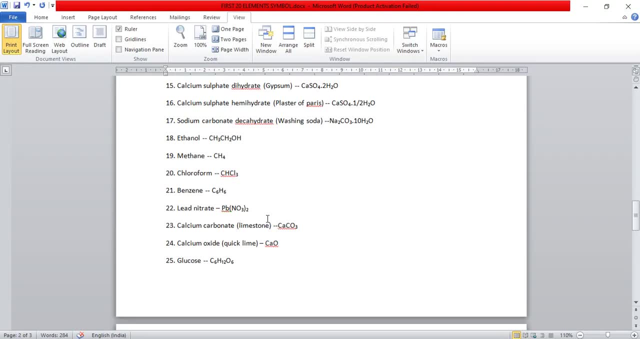 What is the formula of this? benzene, C6H6.. Lead nitrate: The formula of lead nitrate is PbNO3, whole 2.. Next one is calcium carbonate, that is, limestone, The chalk marbles. these are the forms of this. 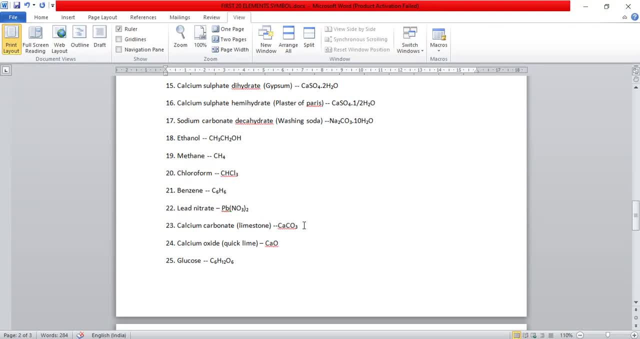 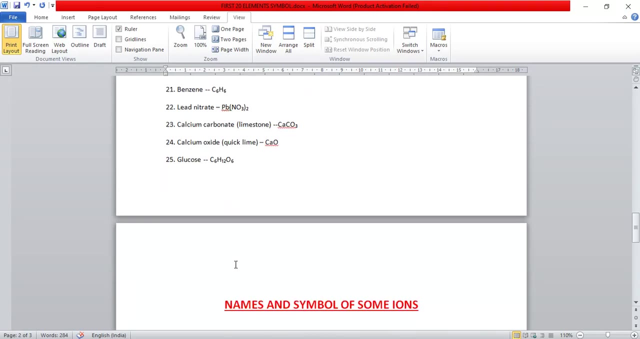 limestone. The formula of this calcium carbonate is CaCO3.. Next one is calcium oxide. What is the formula of calcium oxide? CaO? It is also known as quicklime. The common name of calcium oxide is quicklime. Next one is glucose. The formula of glucose is C6H12O6. Okay, So these are the 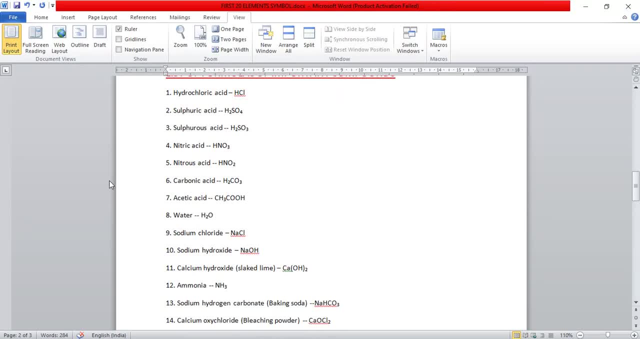 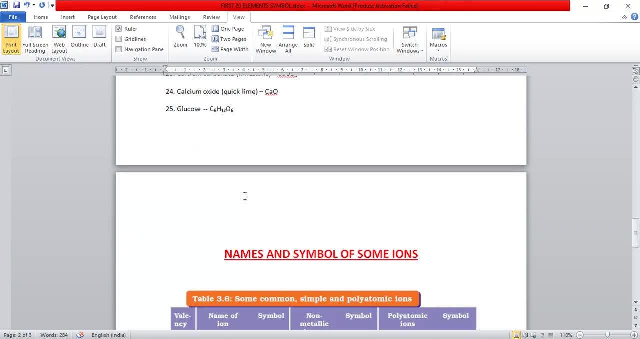 formula. These are the important compounds whose formula you should remember. Okay, You should write like this only, and you should remember the formulas So that you can write each and every reaction. Now we will discuss the names and symbols of some ions. The first of all you should 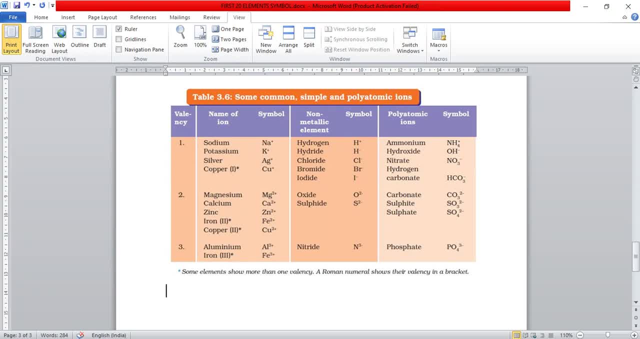 know what is the definition of ion. Okay, What is the definition of ion? Ion, Positively or negatively charged species. Yes, So the ions are group of, are atom or group of atom which contain a positive or a negative charge, Either due to gain of electron or due to. 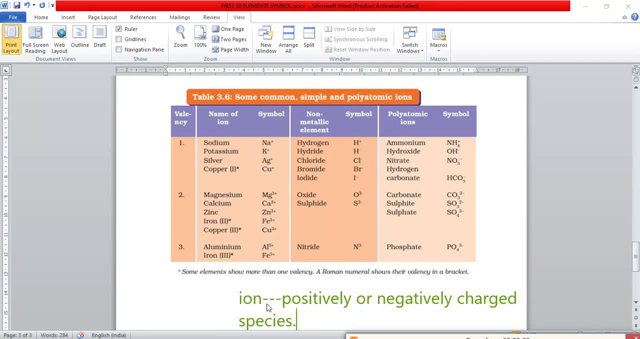 loss of electrons. Okay, So what is the definition of ion? Ions are the atom or group of atom which contain a positive or a negatively charged, either due to gain or loss of electron. If they will lose their electron, they will get a positive charge. If they will gain electrons, they will have a 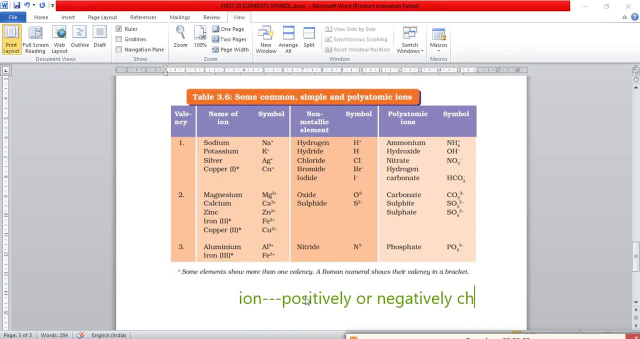 negative charge. Okay, Now we'll see the some of the important, some common, simple and polyatomic ions. formula: sodium: okay, the symbol name of the ion is sodium. the sodium ion can be represented as na plus atomic number of sodium is 11. we'll write: the electronic configuration is 2 comma 8 comma 1, how many electron it has in the 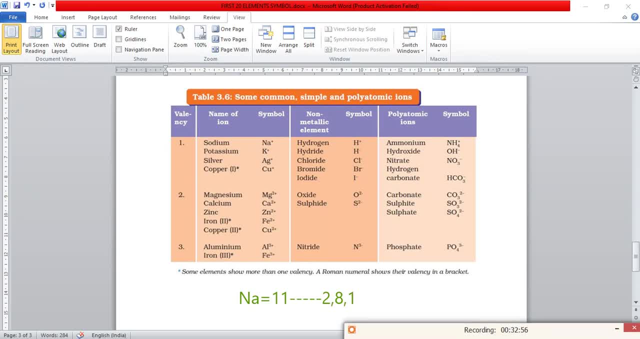 outermost shell. only one electron it has in the outermost shell. only one electron it has in the outermost shell. so this one electron it can donate and it will become na plus okay. likewise potassium: it has a charge of it plus plus charge. one plus charge. 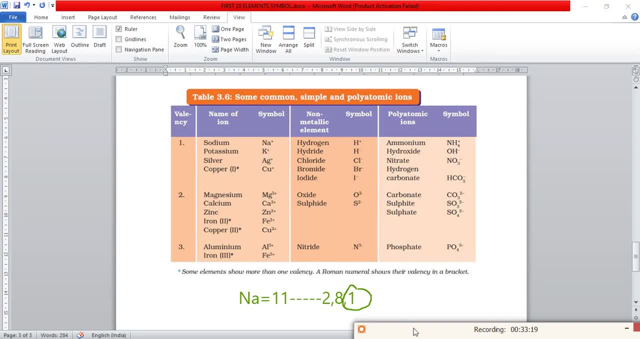 potassium ion can be represented as k plus. so so next silver: it can be represented as ag plus. copper can be represented at cu plus. so these are all our metals, because they can donate their electrons: sodium, potassium, silver, copper. next one is magnesium. magnesium has atomic number of: 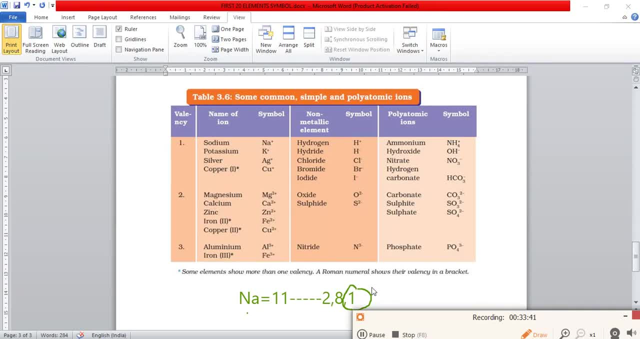 12. they have it. they have atomic number of 12 mg. electronic configuration: two comma eight comma 2, eight comma two means in the outermost shell, how many electrons are present? two electron, this 2 electron, this magnesium can donate and it can become mg two plus. 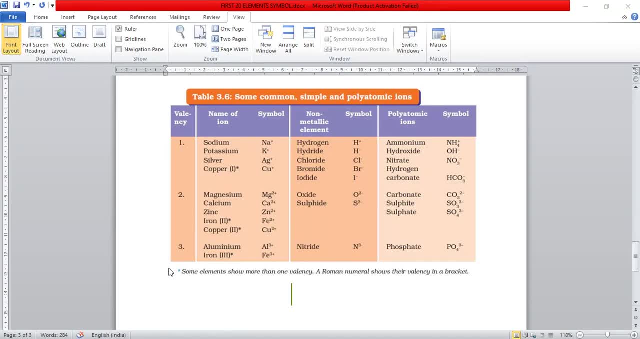 okay, likewise calcium, atomic number 28. it also has to electron in the outermost shell and can donate its to electron to become ca2 plus zinc also has two electron in outermost shell. it will also donate its 2 electrons. it will be positive. mga more ambulance well downtest. 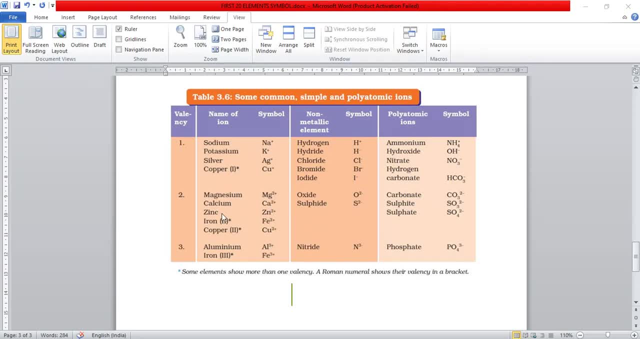 you can love it with the use of this two å sure, this atom is a very powerfuliding, awesome Kız grandfather shreddediman matureそう, not to be cattle. in fact, in the outermost shell in can tonight its two electrons have two electron to become ca two plus zinc also has two electrons- outermost shell it. 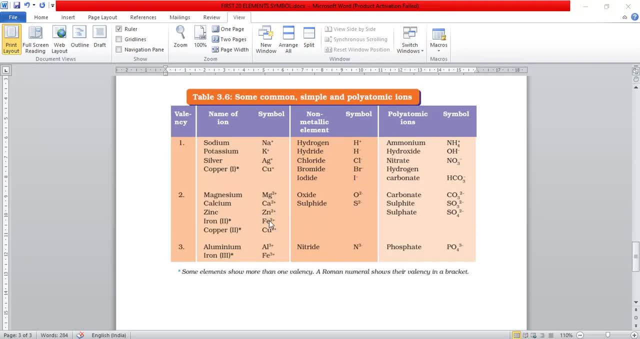 it will become Zn2+. Iron can be represented at Fe2+ Iron, 2 iron. Fe2+ means it has donated 2 electrons, So iron has written as Fe2+. Next, copper. What is the symbol of copper? Cu, Cu2 is. 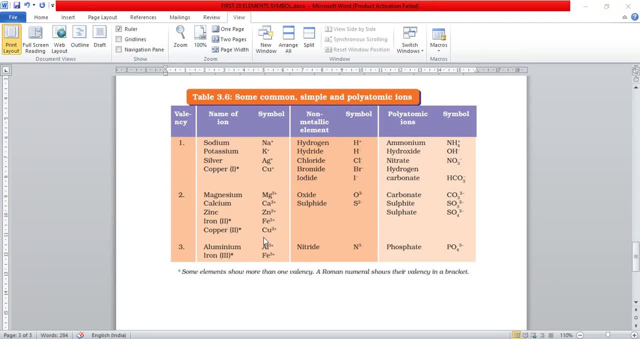 written: Okay, So it has donated its 2 electrons and became Cu2+. Next one is aluminium. The symbol of aluminium is Al. What is the atomic number of aluminium? Yes, 13.. Electronic configuration: 2,, 8, 3.. How many electrons are present in the automotion? 3 electrons. So this 3 electron 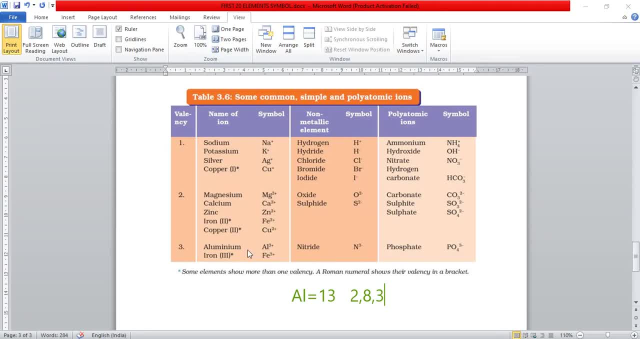 aluminium will donate and it will form an iron, Al3+. Next one is Fe3, means it has donated 3 electrons, So it can be represented as Fe3+. Next one is hydrogen. H+ Means hydrogen only has one electron in its shell, So it will donate its one electron. it will form H+. Okay. 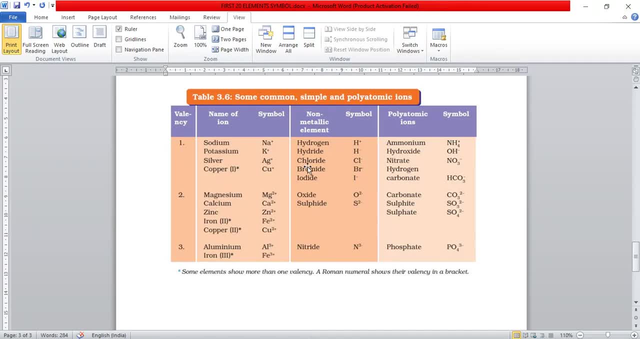 Next one is chloride iron. Chlorine also has one electron in the outmost shell and it will also form Cl- Bromide will form Br- Iodide iron is I- Oxide. O2- Sulfide is S2- Nitride is N3-. 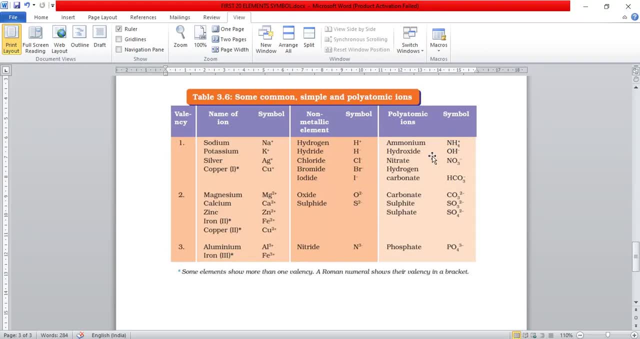 Ammonium iron can be represented as NH4+ Hydroxide iron, as OH- Nitrate, as NO3- Hydrogen carbonate, as HCO3- Carbonate, as CO3- Sulfide, as HCO3- Nitrate, as NO3- Hydrogen carbonate, as HCO3- Carbonate, as CO3-. 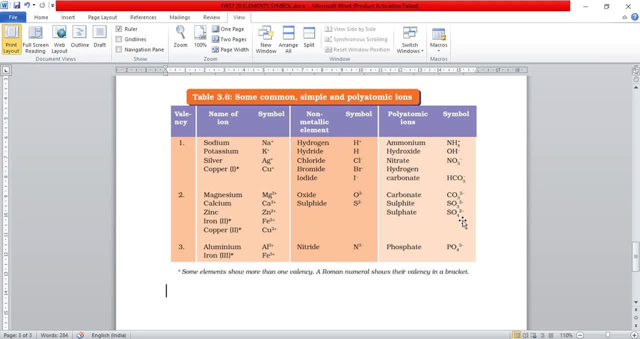 Phosphate as PO4-. So you should remember the formulas of these ions so that you can write the formulas of any compound. Suppose we will see with one example. Suppose we want to write the formula of sodium chloride. So what is how we can represent the sodium ion? Yes, Na+ and chloride. 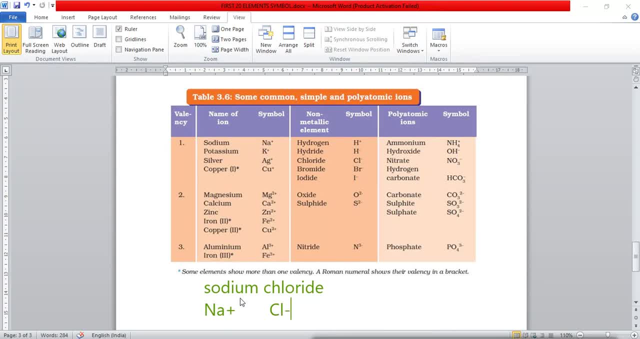 chloride ion can be represented as Cl- So what they will do? They will combine with each other and they will form NaCl. The positive and the negative charge will cancel out their effect and means. they will become neutral and they will form a compound.